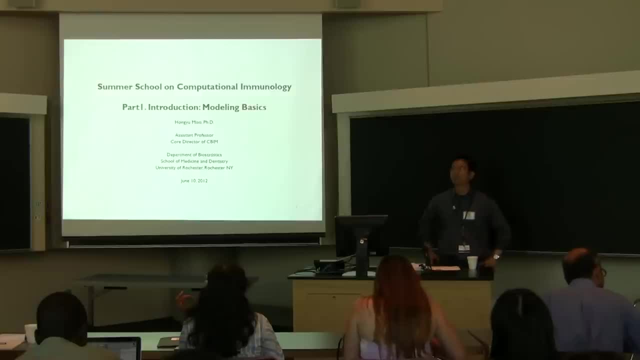 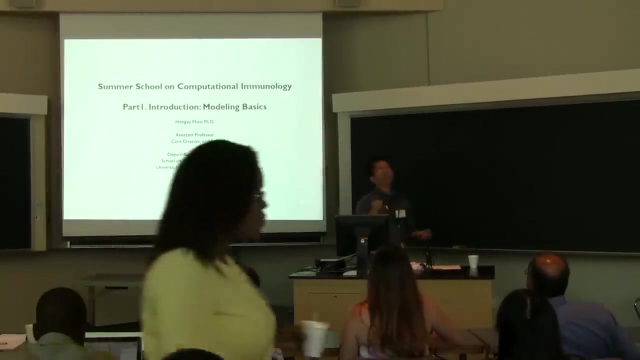 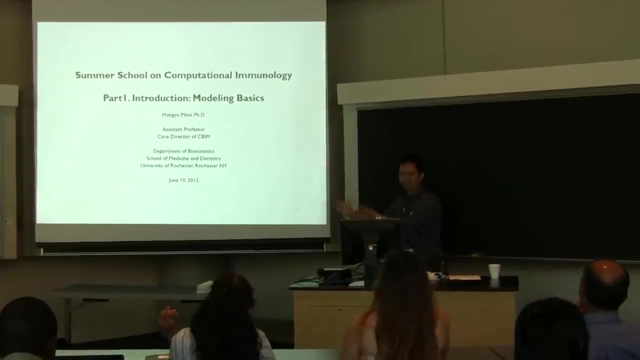 And I believe that, after the talk of Dr Hu and Martin Zhang, you are all right now, fully motivated. right, You are ready to do some modeling, right? Okay, So let's do it. But instead of using languages or diagrams, we start to do modeling using mathematics. So that will be the purpose of the lecture this morning. 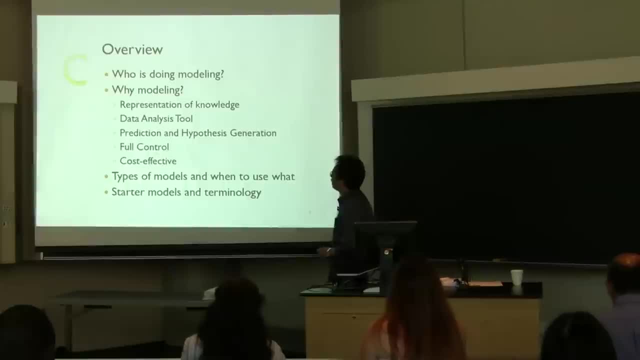 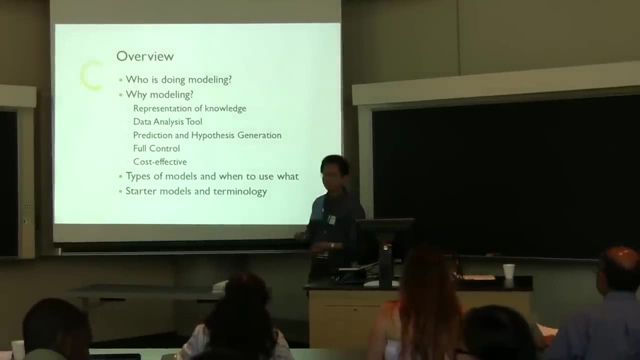 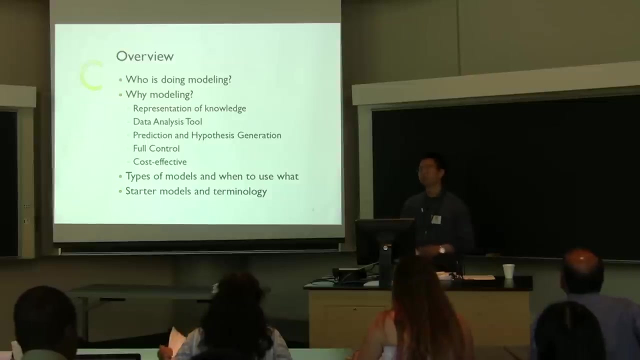 So first, actually, I would like to ask the question: who is doing modeling? Of course, mathematicians, right, Engineers. We do that every day. How about the immunologists? Actually, my personal opinion: okay, You are also doing modeling every day because you are using mice to study humans, And many times that's by leap of faith. okay, Because we just believe that what we learn from the mice actually can be applied to humans. okay, 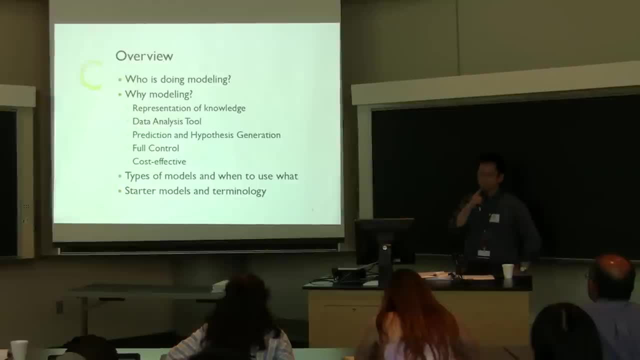 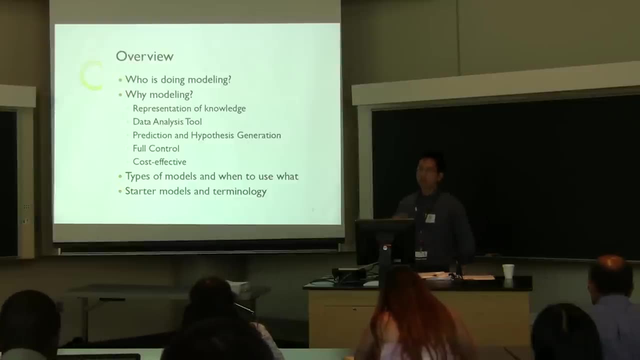 Okay, So So that's modeling. So what is modeling? My understanding, modeling actually is just approximation. okay, It doesn't really mean modeling has to be mathematical or what. So modeling itself, by definition, my understanding, is just approximation. So when we're doing modeling, what will be the benefits we can get? 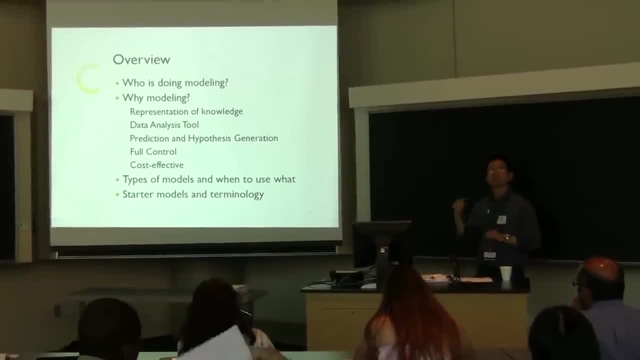 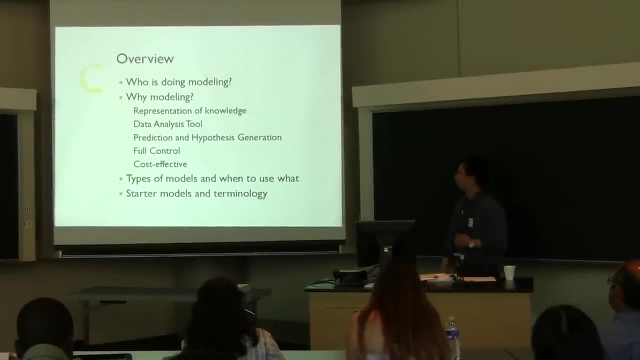 First one: modeling itself is another way to represent our knowledge. I will actually have examples for each of the bulletin later, So for now let's just go over all the points first. So second one: you can use it as a data analysis tool. 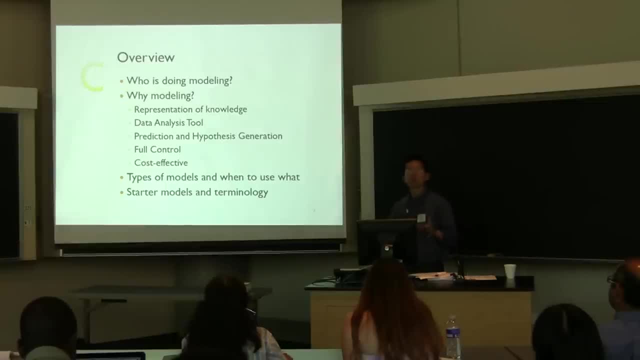 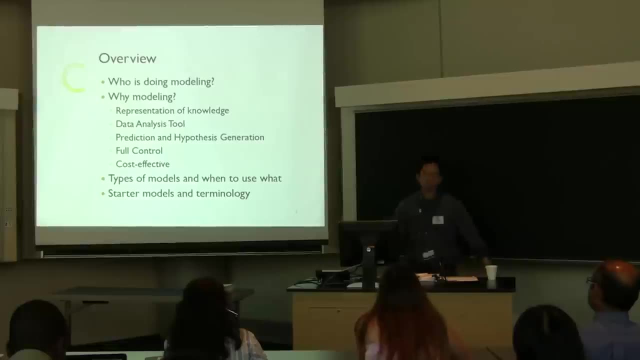 You know that right now, one lab actually can produce 10 times of the data than 10 labs can produce in the past. So, within this huge bundle of data, you need to find a way, a systematic way to describe them, organize them. 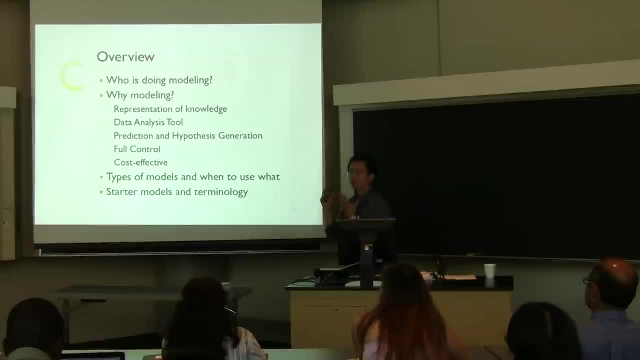 And eventually you want to extract useful information from this data. So that's what model can help. Also, you can use the model to do a prediction and generate a hypothesis. Sometimes I find that's actually quite easy if I do that using model. 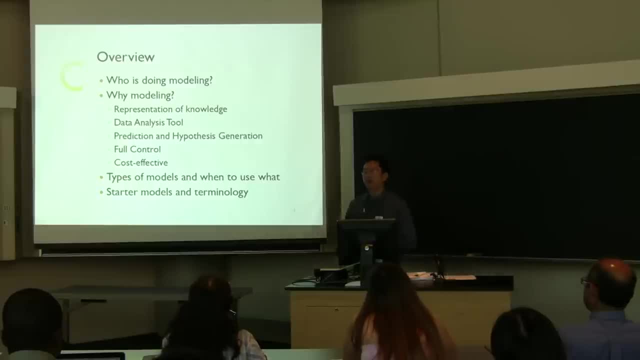 However, in experiments it's not easy. sometimes, For example, I can actually change the number of web cell cells in the lung so that I can actually look at the effect of available target cells on the virus infection. But I can do that in the model, just change the number. 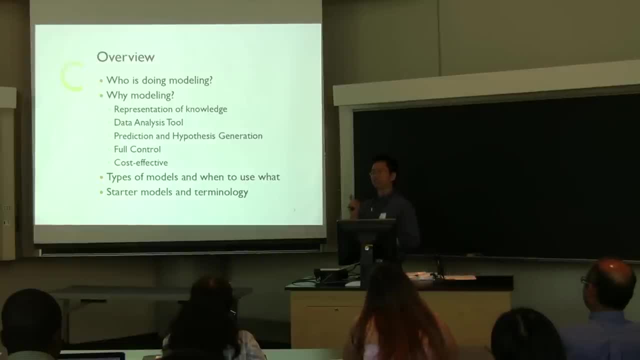 But you may not believe the results. I have to say that in advance, But it doesn't matter. We have a bunch of ways to check our model and to check our results, which that's something I'm going to talk about later, actually tomorrow. 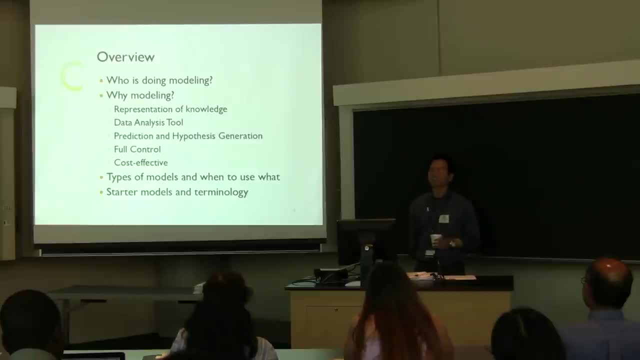 Today I only have three hours, one hours in the morning, two hours in the afternoon, And I don't really have that much time to talk about all the details, but for now it should be OK. So the fourth thing is we have full control of our model. 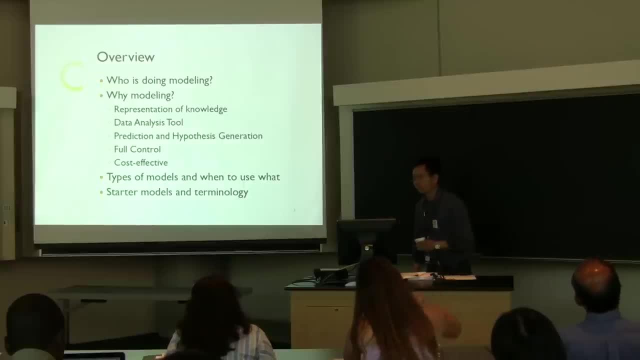 because you created it Right. You know every detail about the model. It's not like a biological system. Even you design the experiments. you know there are many factors. we don't know What's the role they're playing, For example, cytokines. 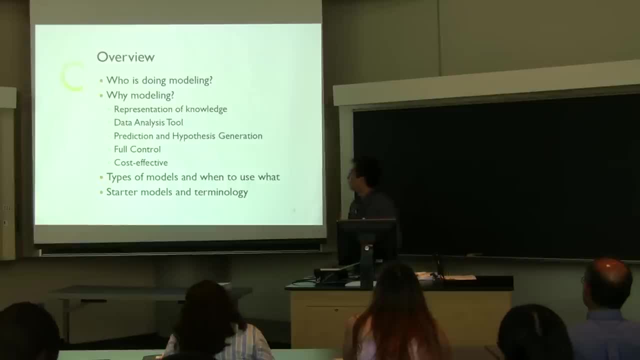 OK, what's the roles of all cytokines in the immunity? We haven't fully understand yet, But for the model you already have this advantage because you simplified the problem. You approximate the real problem. So last one is cost effective. 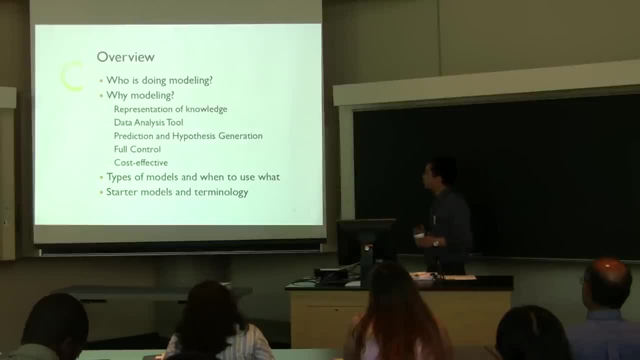 So by saying this actually, I mean we can actually use computer simulation to help to design experiments and generate hypothesis and find out the most promising direction for new experiments. So instead of randomly trying the combinations- you know there are an infinite number of combinations- 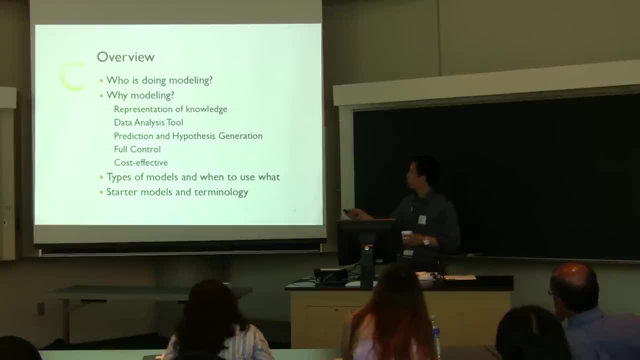 you can try in experiments, But the models Sometimes can give you some clue. So also we're going to actually learn the general types of models And, more importantly, we're going to use what type of models. So models are like your culture for ICs. 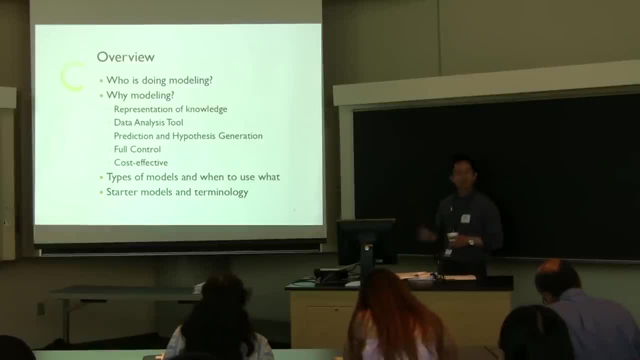 It doesn't mean one IC can matter everything. Different types of models. you have to choose different types of models to solve different types of problems. Unfortunately, in the summer school we're going to only learn- mainly we're going to only learn- the ODE and the ICNB model. 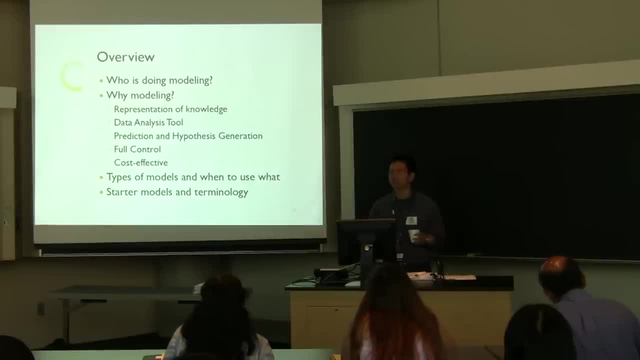 But there are actually tons of different models you can use in practice. Also, at the end of this lecture we're going to learn some very simple models and get familiar with the terminology so we can be prepared to do modeling. So back to the example. 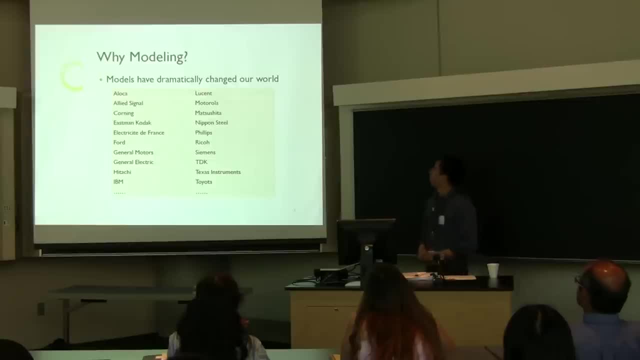 OK, Here is actually the name I put from a web page. That's big companies. You know what a company is? right, They're actually doing modeling every day. For example, a car company. When they design a car, they actually 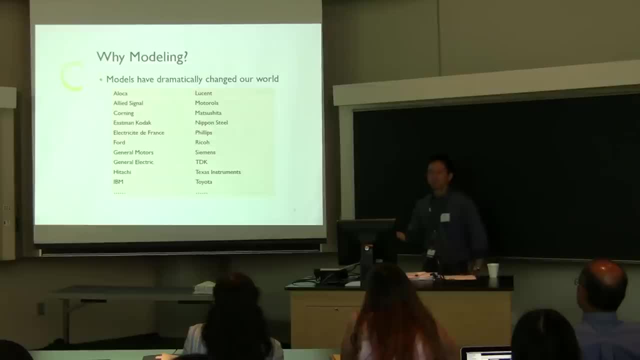 start to do modeling at the very beginning, Before they actually crash the car in the lab. they actually crash the car tons of times in the computer first, So that's how they come up with the optimal model Structure. That's why they can actually evaluate the safety beforehand. 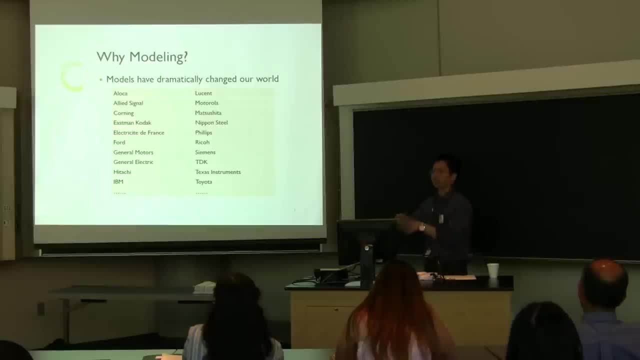 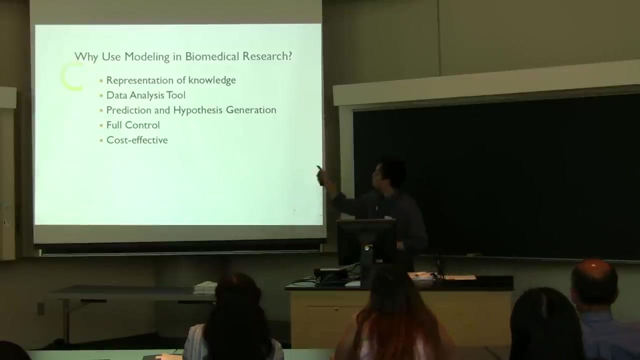 Instead of designing some defective cars and then later you change the design. That will be too custom. So here's just some example. Second one: I want to talk about why we use modeling in biomedical research. So I have an example for each of the five points. 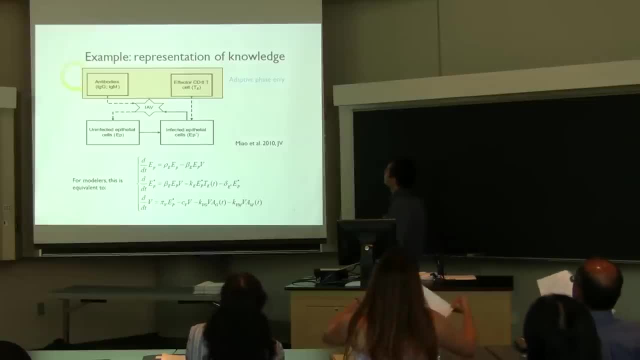 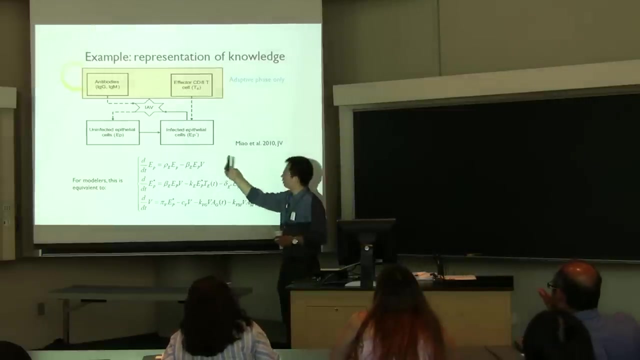 The first one. This one is a representation of a knowledge. So I think that we all have a problem with diagram right Diagram actually show us the infection or dynamics, What's going on in the lung after a primary influenza virus infection. This part we have a pointer. 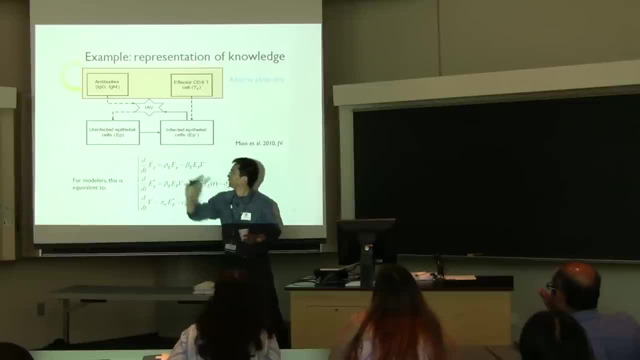 Anyway, I cannot find pointer. OK, This touch. So this one is actually our target cell. It's a cells in the lung And this is an infected cell, And we know that during the adaptive immune response stage we have antibodies in fact kicking. 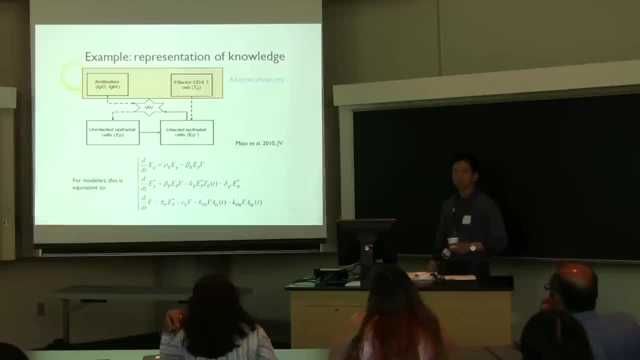 And also the effect for CDAT cells will play a role By actually drawing this kind of arrow. OK, you can see a direction. This direction is from uninfected cells. It can become infected due to virus, OK infection. So the diagram pretty much explains the story, right. 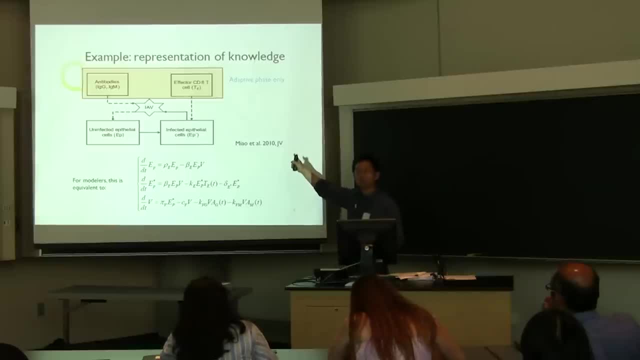 By looking at the different components and the direction of the arrows. However, if we just do it in mathematics, OK, this actually is really quick. It is telling the exact same story. OK, here We are actually just using a different language, OK. 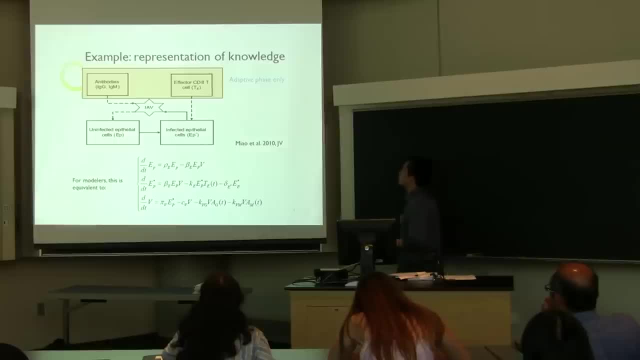 The biology is the same. So in that sense, OK, I would say, sometimes you can actually use mathematics modeling as a tool to represent your knowledge. OK, That's fine. Once you know what's this language, OK, you will be comfortable with this language. 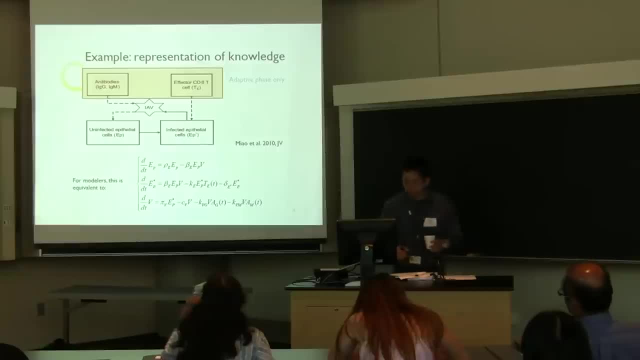 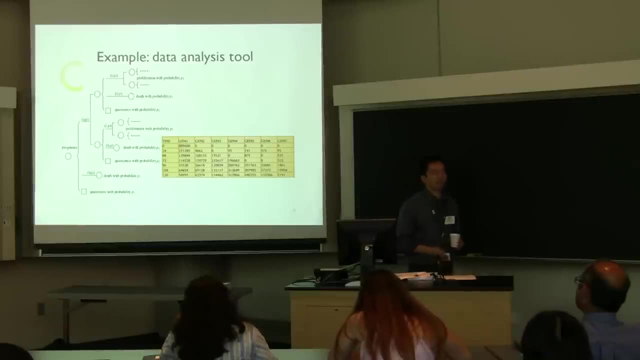 like you are comfortable with the diagram. So the second example is that actually Martin already talked about the CFAZ data analysis, right, And instead of a OK Part of the marker intensity, OK, I just put up a number here, OK, 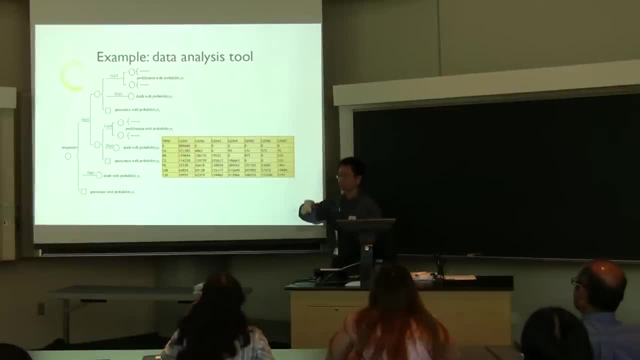 Because eventually- not eventually- you can actually skip some steps. Anyway, this is data you can get from the CFAZ labeling. At different time points you can get a number of cells in different generation. Here generation means the number of division. 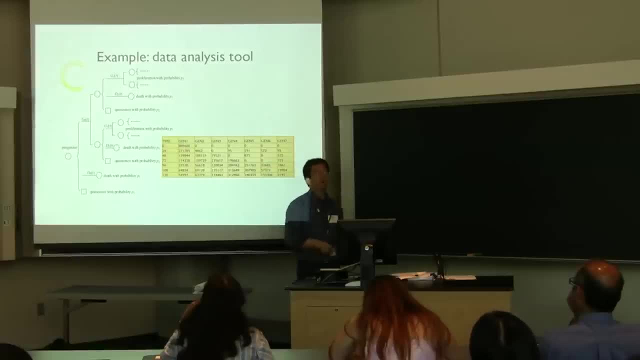 For example, there's generation one means these cells never undergo any division. OK, During the time window of experiments, This one is after one division. OK, So you have this kind of experiment results. So can you actually ask the same question as Martin just asked? 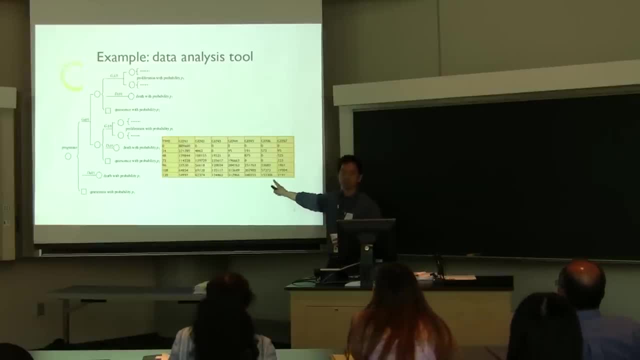 Can you actually tell the time to division or time to death just from this data? It's not easy, because this data just tells you the number of cells at different time points. right, And how do we know? OK, that the number of cells, the number, 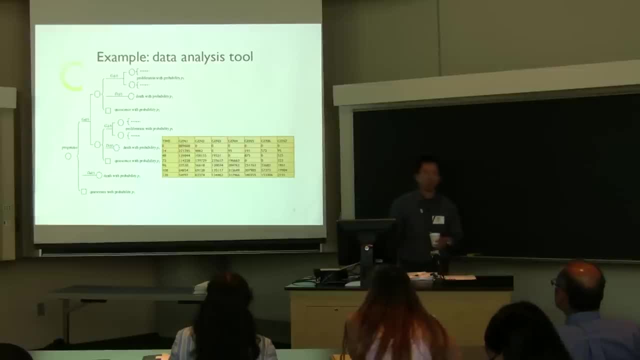 of cells, Right Right. And how do we know the average time to division or time to death? So that's where we can actually use the mathematical models. This actually is a schematic illustration of the mathematical models we actually use to analyze the data. 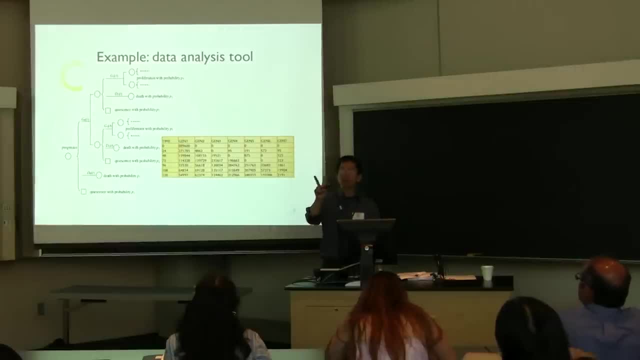 By using this data, actually, we can figure out that the two parameters are interesting. OK, Time to division and time to death. And under different stimulation- OK, that's probably what we're really interested in. Under different stimulation: OK, what will be the change? 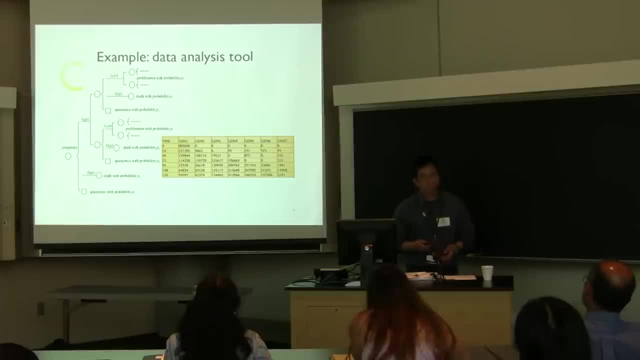 in that time to division and time to death, right? Are those numbers here in generation four, five and six? those zeros are those, Yes, You're supposed to, After the 572, then you have 0,, 0, and then you have more. 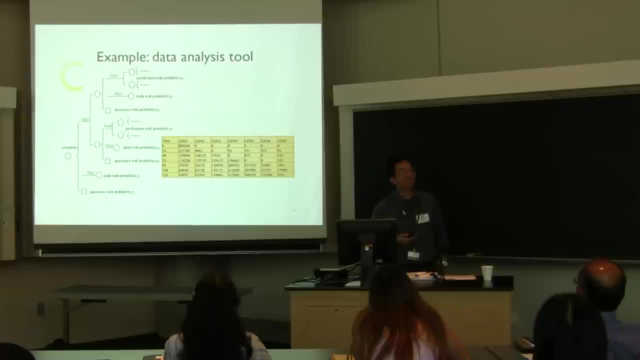 So are those Noise Noise? OK, So can you just take them out on your model. If I have an error-free system, OK, I would expect that I see zero here, see all zero here, All zero here, all zero here, because there is a delay. OK. 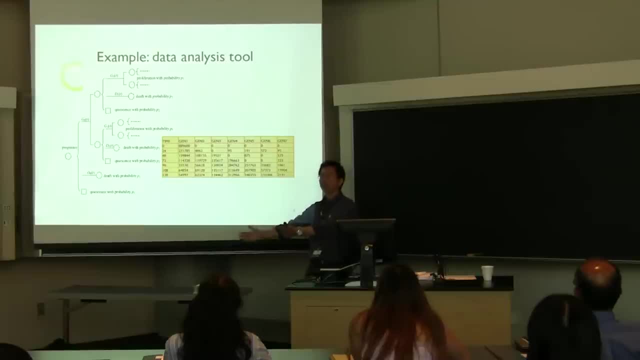 You need time to finish the first division and then finish the second division, right? However, with error, you'll get a. this is a real number, OK, That's why you get an error here. So Now something doesn't work. 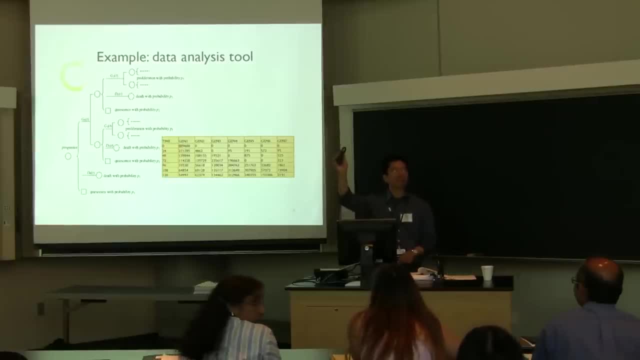 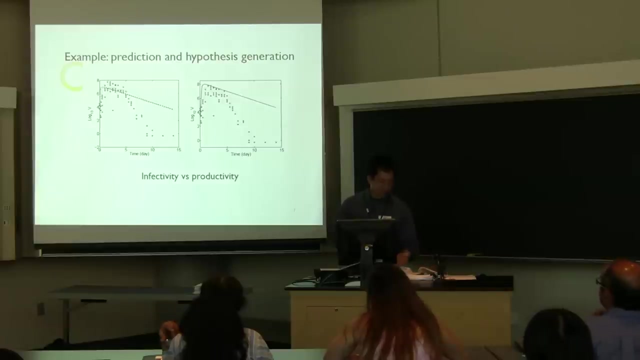 Gene, I got a warning sign Battery's out. That's why, OK, I'm going to use the keyboard anyway. So the third example I want to talk about actually is how to use a model to do prediction and generate. 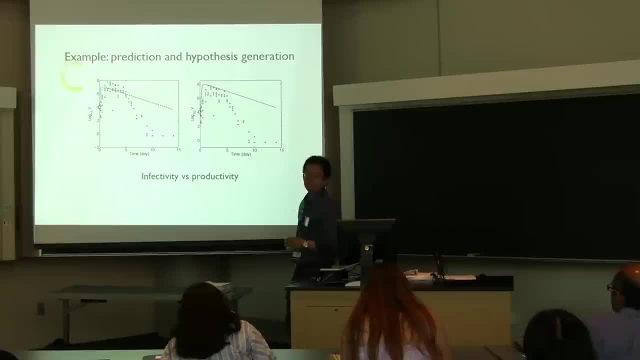 hypothesis. For example, let's consider a new influence, hours a spring, OK. What we actually want to answer is that if a new influence with high infectivity OK, but moderate productivity OK, will this strain be more dangerous than a strain with? 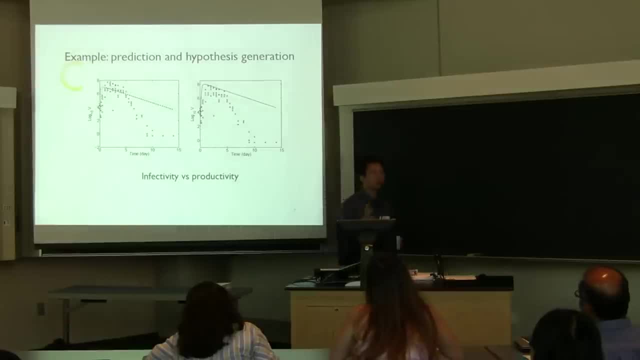 moderate infectivity but high productivity to infect the individual. Of course I'm not talking about epidemics, OK, So we actually did some, you know, simulation based on the model we have And surprisingly OK. we had thought that infectivity should. 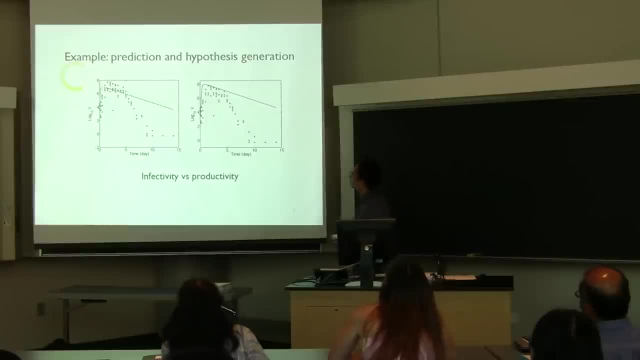 be the key factor. But later, when we look at these plots, if we change the infectivity- OK, actually for a few orders of magnitude, OK, the viral load peak, actually almost the same, remains almost the same. So, which means if I increase the infectivity of virus, it 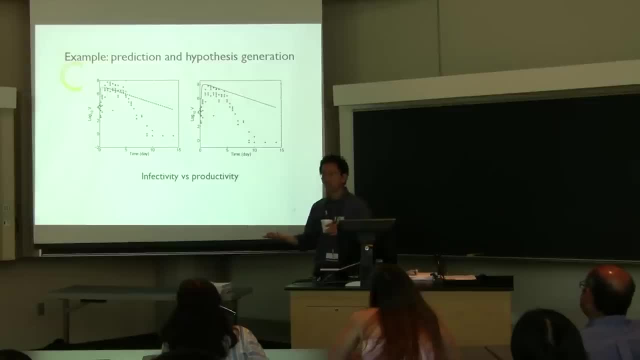 only exhausts our target cell pool earlier. OK, And they cannot actually produce more viral particles- OK, within the primary infection. However, if I just increase the productivity, OK, for a few orders of magnitude. what you see here? the peak of the viral 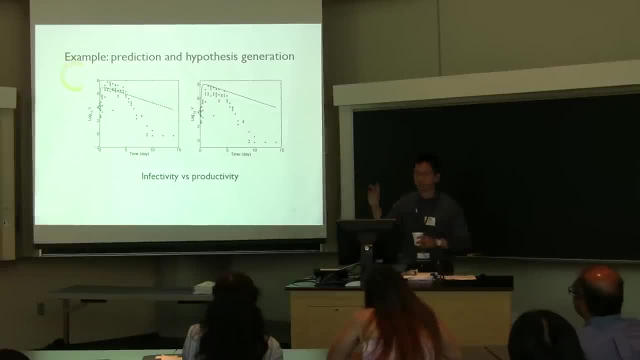 load actually changes a few orders of magnitude, So that's something OK. some simple example: Once we have the model, have the pump values, we can simply, you know, manipulate the pump values to see what will go on OK with the system. 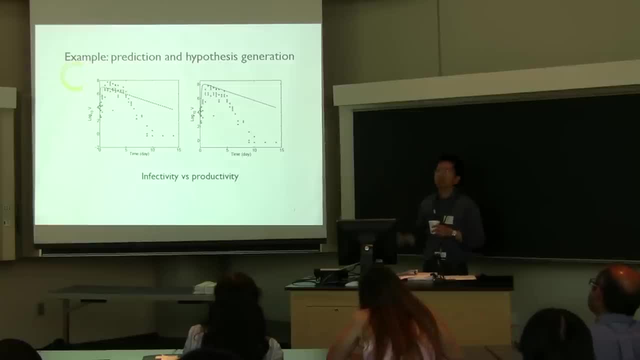 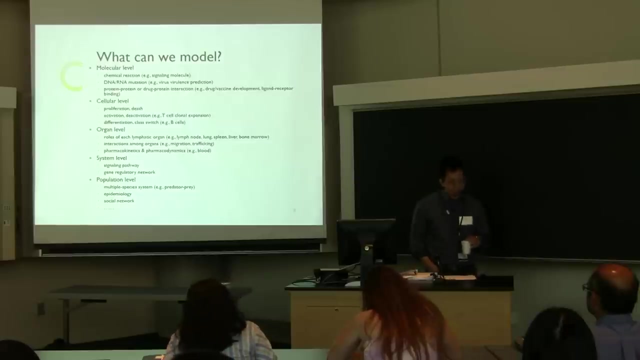 And this is a prediction, And actually you can match this prediction with H1N1, OK, behavior, OK. That's exactly the example, OK, of the prediction result. So now, after we know, OK, what the models can be used for, 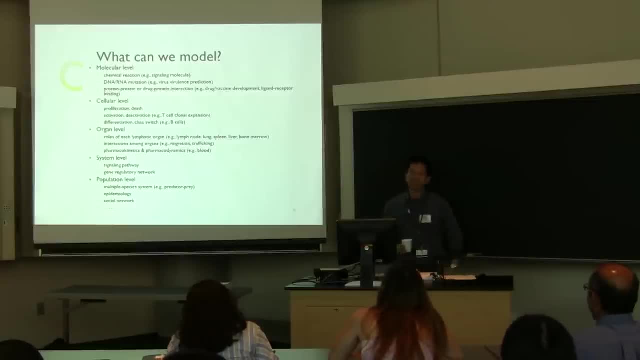 now let's look at what actually we can model. OK, So, like I said, we have the H1N1.. We have the H1N1.. We have the H2.. We have the H3.. We have the H4. 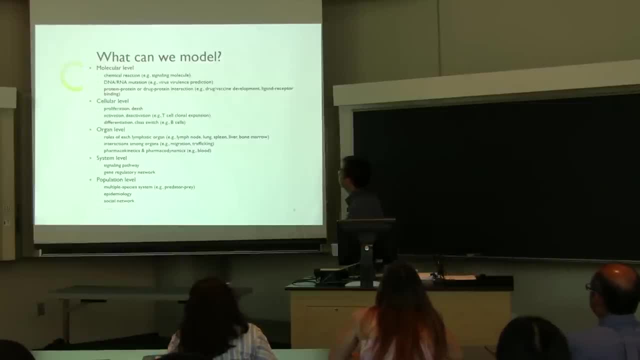 We have the H5., We have the H6., We have the H7. So, like just mention before, there are tons of things we can model At the molecular level. you can model the chemical reaction, For example the interactions between the signaling molecules. 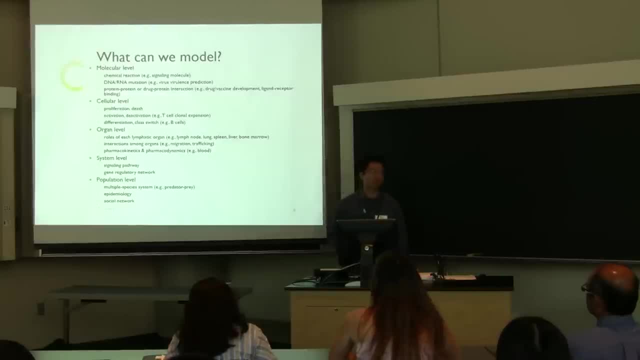 OK, by doing molecular dynamics. OK, if you know something about molecular dynamics, you know you can use the AMBR many packages. OK, That's good simulation. And you can also model the DNA remutation, For example. you can use this kind of thing to predict viral. 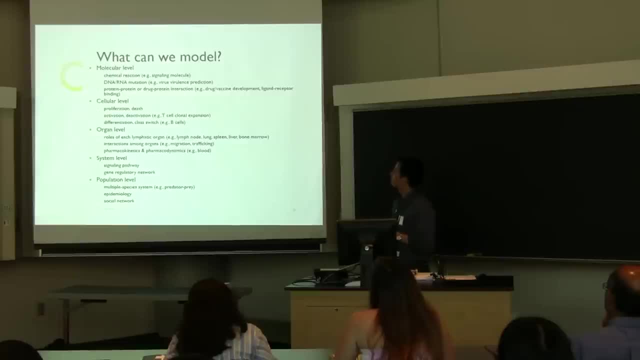 violence And also- you can also do this, OK, of course- model the protein-protein interaction or drug-protein interaction At the cellular level. of course we are interested in the perforation bias. that kind of rates right. 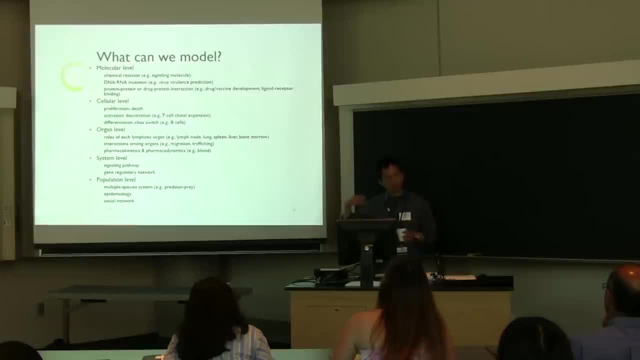 Because under many circumstances, in that there's lots of information And activation, deactivation and the differentiation class space for B cells At the organ level, you actually compare the contributions of different lymphatic organs, For example the lymph node, the lung spleen, liver, bone marrow. 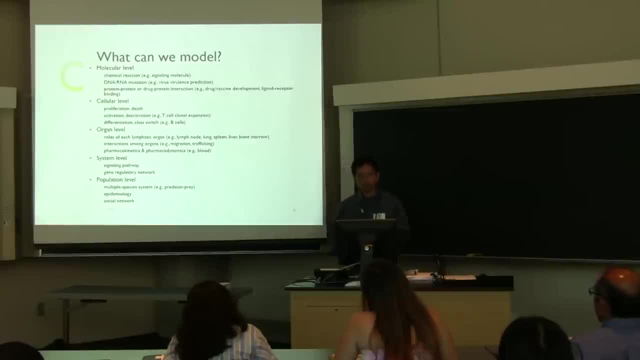 In a recent study we actually compared the contribution of spleen with the contribution of a lymph node. So in essence, you can identify which place actually is the major resource of immune cells. to help you to answer that kind of question Also, we can. 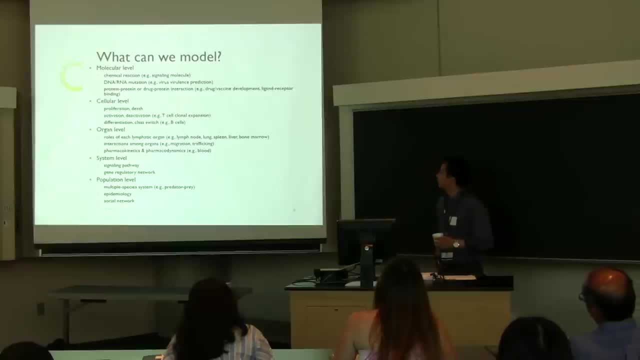 We can look at the TW Alturasome to mechanical interventionary interaction patterns between population cell and chemical cell. If I simply rotate the study and then look at the differential, If I look at the, I'm much deeper. Basically that's migration and trafficking. 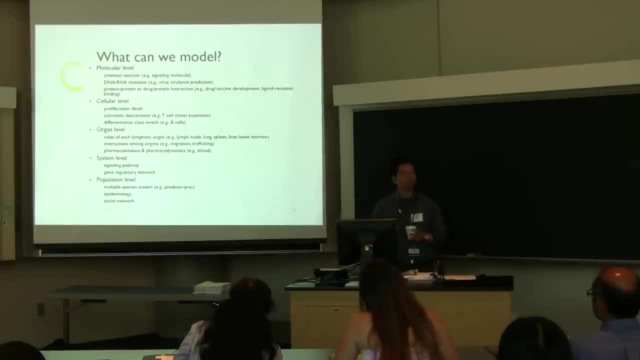 of cells, molecules. Of course, if you are doing PTPD you get aied blood sample. You want to know, because data pattern will usually be up and down. From this up and down pattern you want to infer the rates of PTPD. 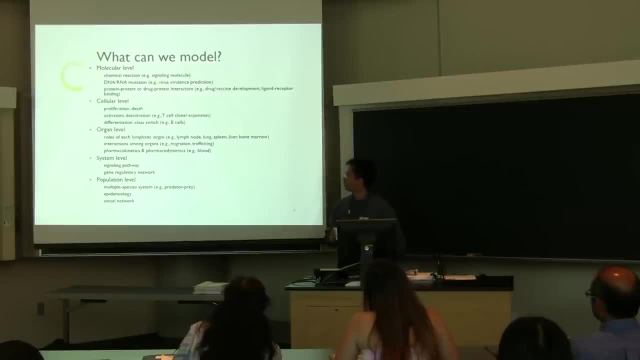 And on the system level, I think that's a hot topic right now. So on that, ichi, people will change. At the system level, people are interested in signaling pathway, metabolic pathway networks and you can do the gene regulatory networks, but of course we know for this kind of larger 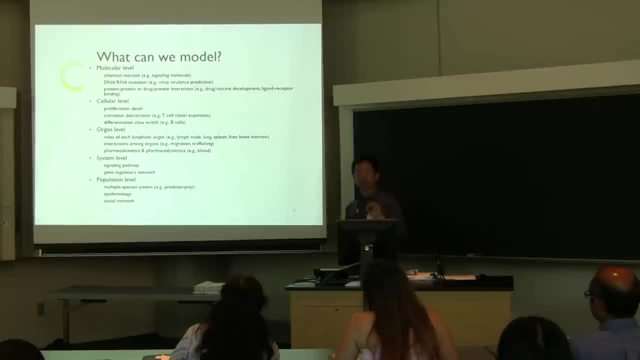 scale model. we also have lots of technique issues and also many inference problems For the population level. we can do a multi-species system, like the simplest one is a pre-to-pre system, right, just two variables, two species, And we can do epidemiology, social network, so that kind of thing. 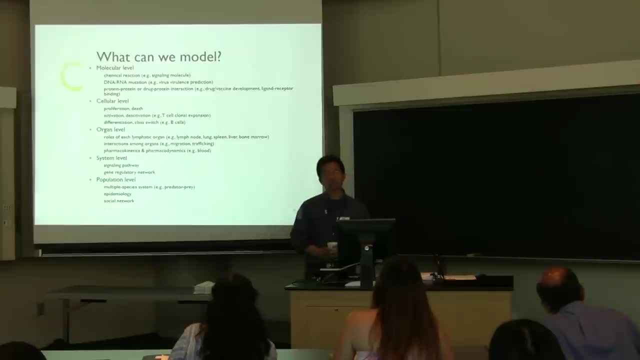 So it sounds like I'm saying that we can model everything and we can do everything. However, I have to go back to experiments. okay, Modeling is just modeling. okay, Whatever results we get or predictions or hypothesis we generate have to be verified. 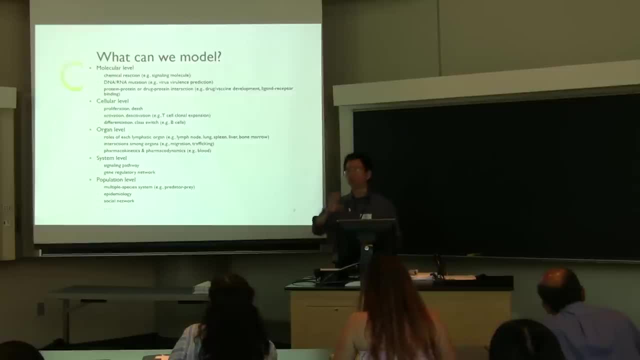 by experiments? okay, I'm not saying modeling. modelers can live by doing modeling alone. okay, Have to do it together. Who is the immunologist? Okay, Thank you. So One question In this perspective: you were telling the prediction and the hypothesis generation. 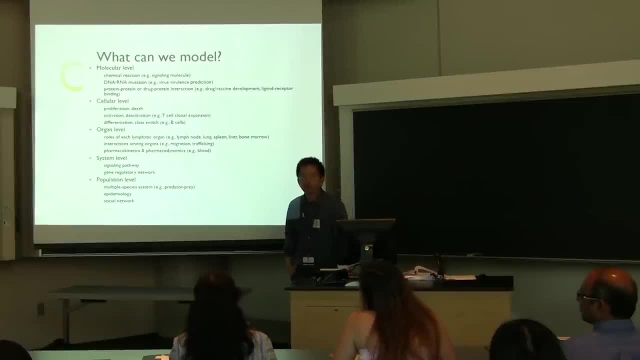 Along with that, whether it is possible to model for experimental validation. So you want to use model to evaluate your experiments? Yes, Like if you're doing, say, for example, studies and further downstream we'll be doing some chemistry or something to do with a selective list of candidate genes. 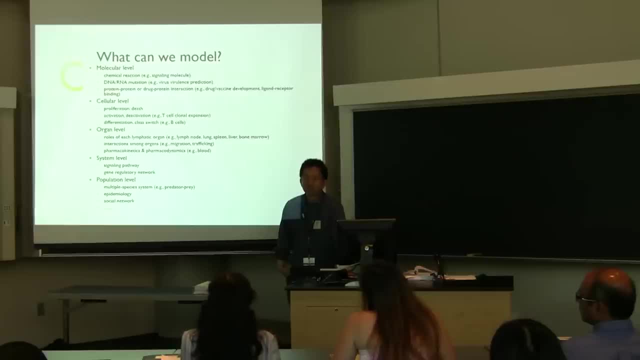 So in such scenarios, instead of going for the Okay, Even on histochemistry or something, Whether we can go ahead with the modeling to just to validate some of the candidate genes, That's possible Because we know that for the thing you just mentioned, okay, many times we measure that. 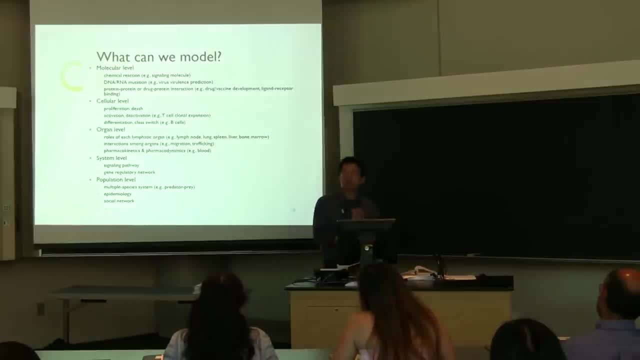 actually is too complicated. We hope that using this kind of a measurement, we can understand the system, but we are not able to directly measure what we want to measure. okay, So in that case we can actually develop a system where we can actually use this kind. 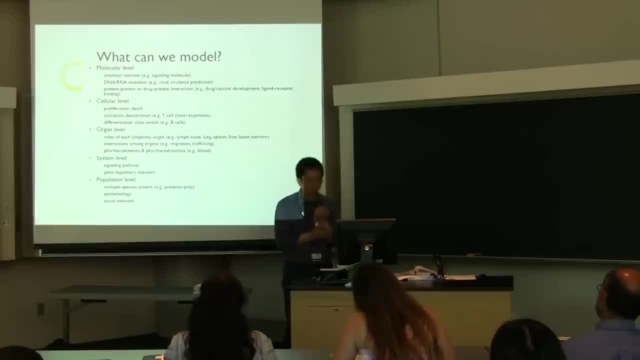 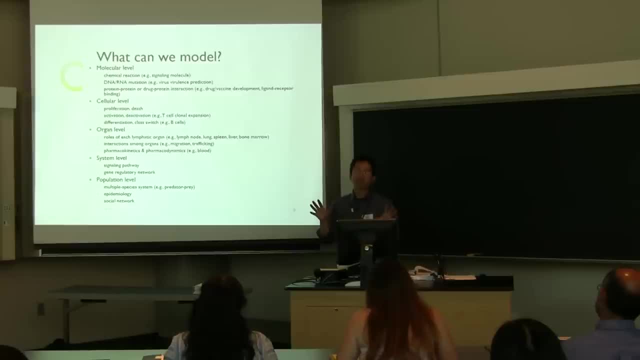 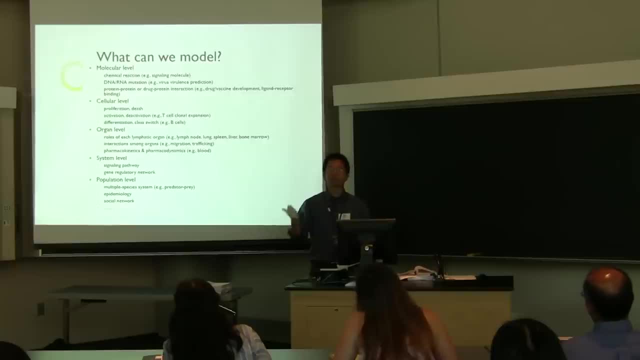 to verify whether one of the hypothesis is the best one or the most accurate one that's supported by data? Okay, But that would be a very general answer. okay, I have to say, because I don't have too much time to talk about the. 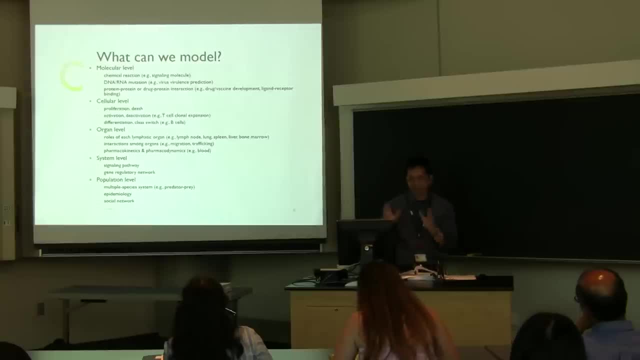 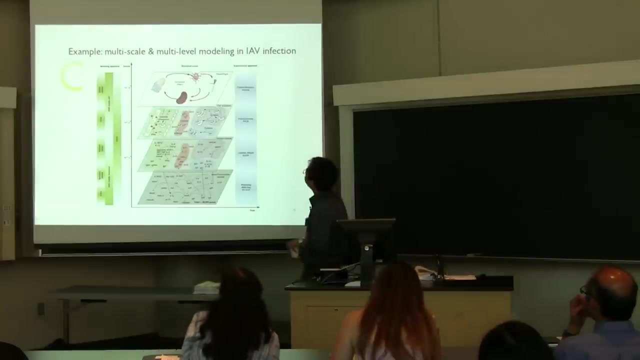 as a concrete example. given the circumstances of the summer school, It's more like education, But anyway, you're welcome to talk to me after the lecture. So here I want to actually give you that's exactly the sort of thing you're interested in. 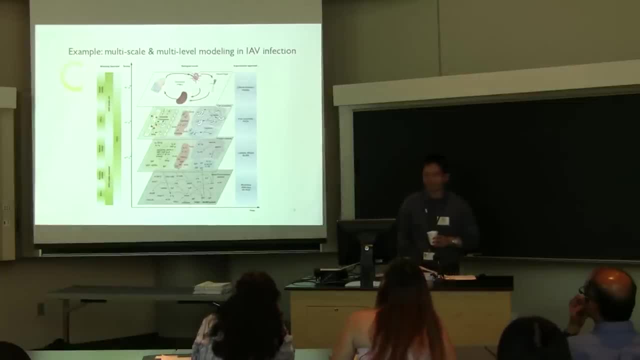 Give you an example of what we're working on. This is a big picture in our mind and we're still working on it, So we want to understand the influenza infection within the past few years and also actually the vaccination and the adjuvant effect in the next few years. 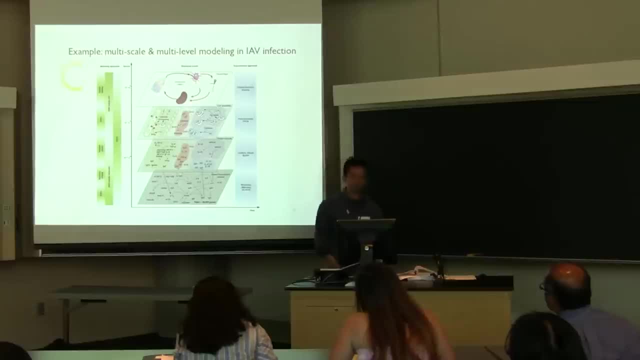 In our mind, we divide this system into four layers. We have a genetic layer, That's the bottom one. We have this protein, This is the molecular layer, And this is the cellular layer, and the top one is the organ. Right now we're not actually really moving on to epidemics. 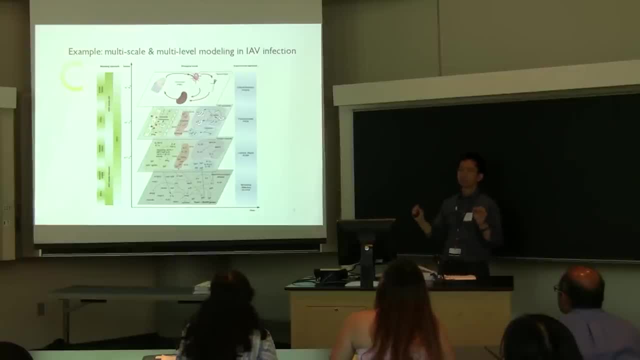 So we focused actually on within-host immune response or vaccination. So at this level you can definitely do some gene-recognitory network modeling And you can also construct a 2D. I call it a 2D or 3D network. 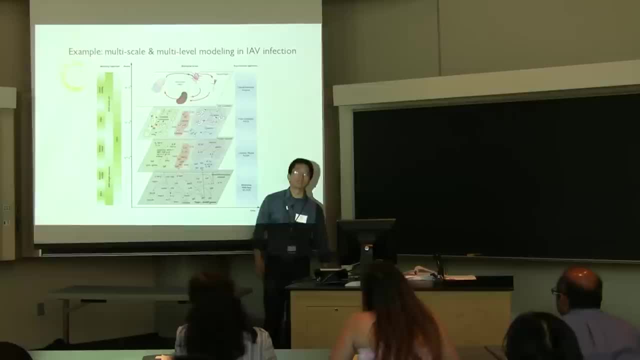 to actually go through this cell count, chemo count, whatever regulation factor, and then back to the gene network, And also we want to understand the cell kinetics. What do they do And how fast do they do something? So that's kind of the question. 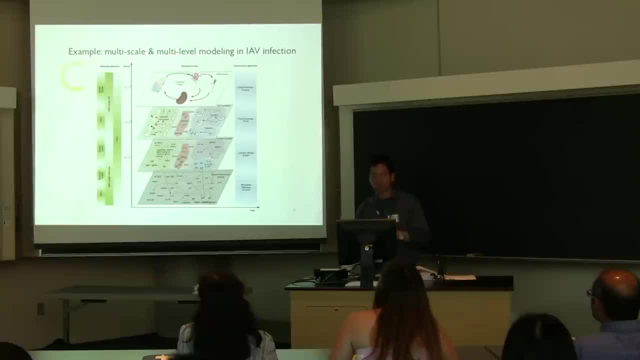 Org network is more like migration interaction, because we know many immunological phenomena actually that are localized Inflammation- OK, They're localized, They're not actually everywhere. So that will be the example. Of course, that's just big picture, OK. 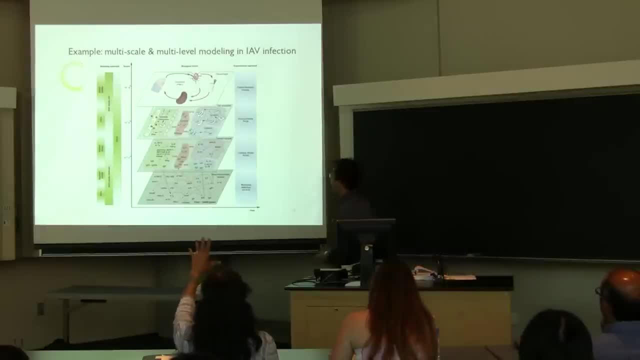 Is this a published one or an unpublished one? We published some papers for some specific problems. For the whole system. it takes lots of resources and time to finish, But I don't think actually we can finish this alone because I think that's the job of the immunologists. 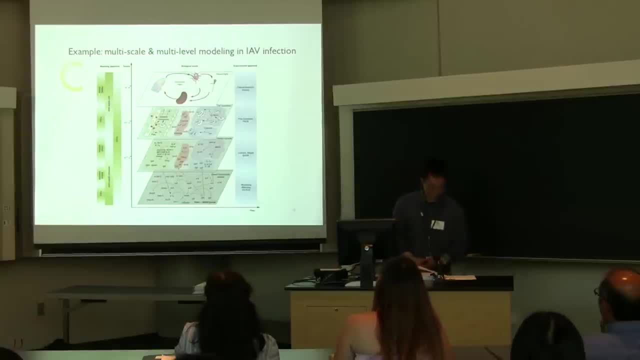 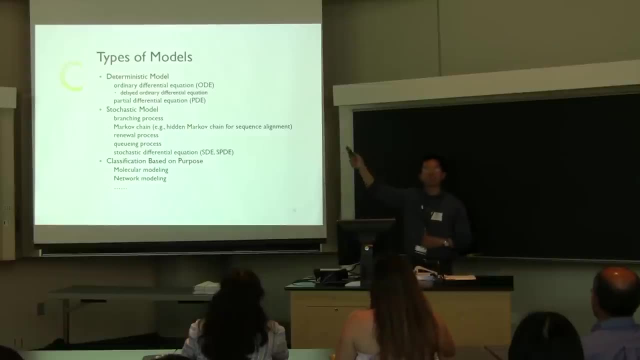 over the world? OK, Not just the one center here. OK, So to model that many different things? OK, what type of model can we use? OK, Here we'll talk about different types of models. So in general, we actually can divide different types of models. 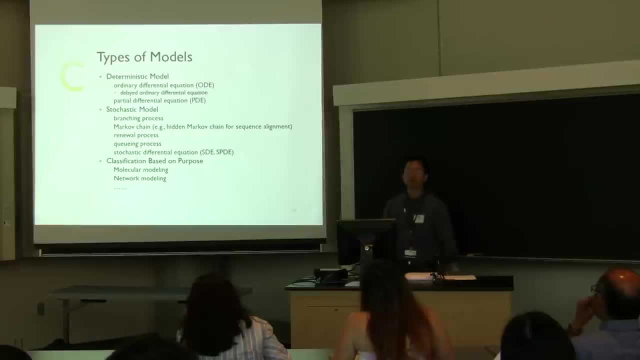 into two categories. The first one is so-called deterministic models. The second one is so-called stochastic model. The so-called deterministic models, which means these models do not consider randomness- OK, That's a key difference. And by the stochastic model, actually, they explicitly 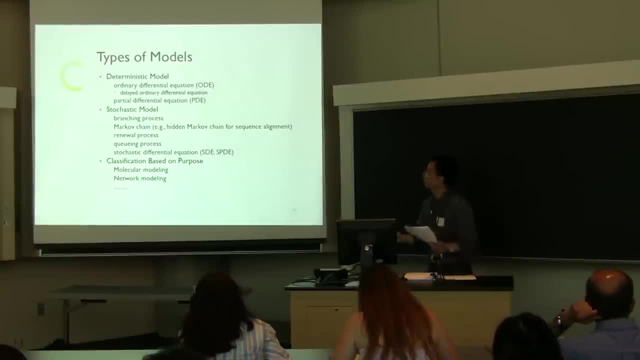 take the randomness into consideration. OK, That's a key difference. So under the category of deterministic model, we have a so-called ordinary differential equation model- ODE OK, OK, OK, And we also have some variation of ODE- OK. 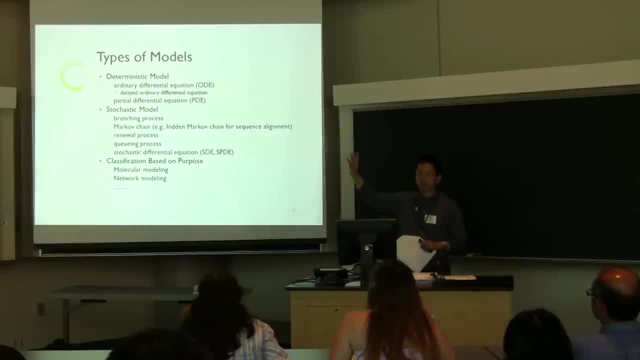 For example, the delayed ODE. We also have something called a PDE partial differential equation. So the difference between ODE and PDE is that PDE is more complicated. That's not a satisfying answer, right? The key difference actually is that ODE only. 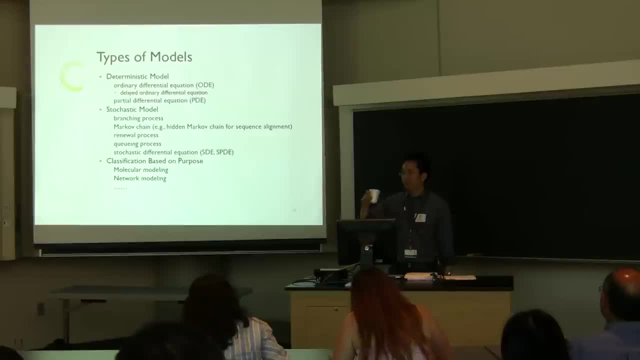 can model a well-mixed culture of particles, which means it cannot consider spatial difference. PDE actually can take the spatial difference into consideration. OK, That's a key difference, But I'm not saying wrong things. OK, PDE is much more complicated than ODE. 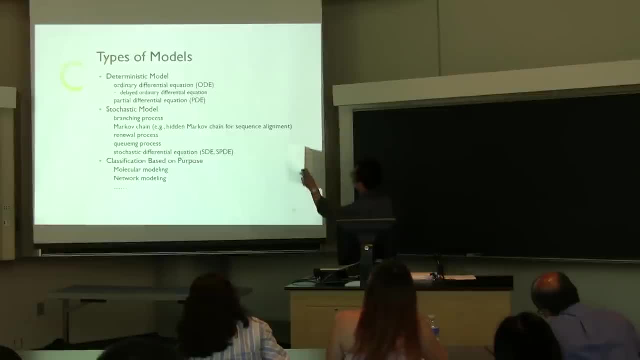 We're going to actually have some example this afternoon to look at these two things. So for the stochastic model: OK, there are actually too many different types of stochastic models, For example, branch processes. OK, We know that it's actually derived from 1950s or 50s. 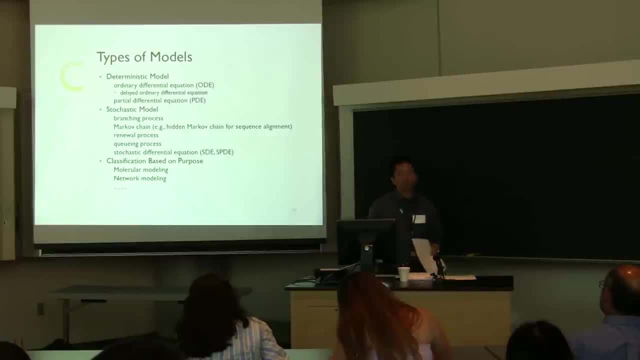 or 60s, 40s, But anyway, that's a long time ago. And people want to use this kind of thing to understand the cell cycle. OK, That's actually. we're going to have an example for this. Also, people use a macro chain or hidden macro chain- OK, 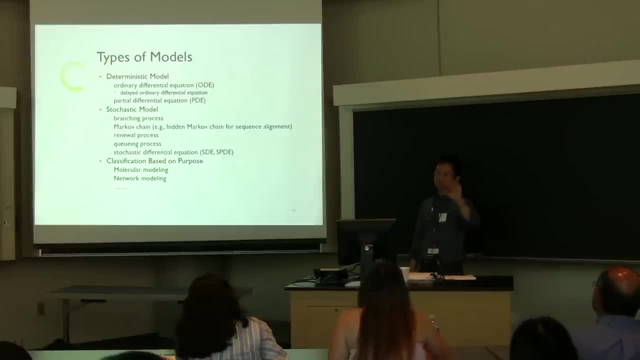 not only to model the cell behavior or cell kinetics, You can also use a macro chain model to model the sequence alignment. OK, if you're using, for example, BLAST or whatever that kind of sequence alignment algorithm. OK, There is a type of tours that actually 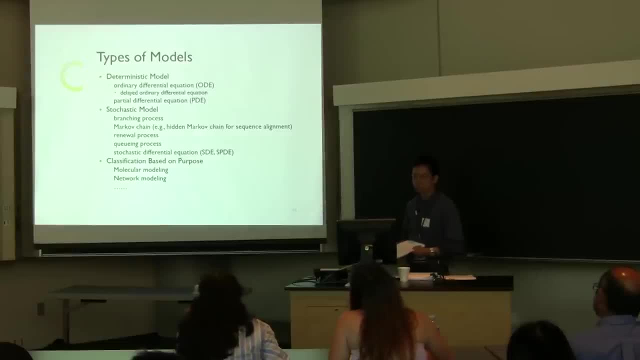 use the hidden macro chain model to do this, And there is something called a renewal process, which means a process can start and end and restart again, So that's called renewal process. OK, Queuing process is more like you have 10 customers go to a bank. 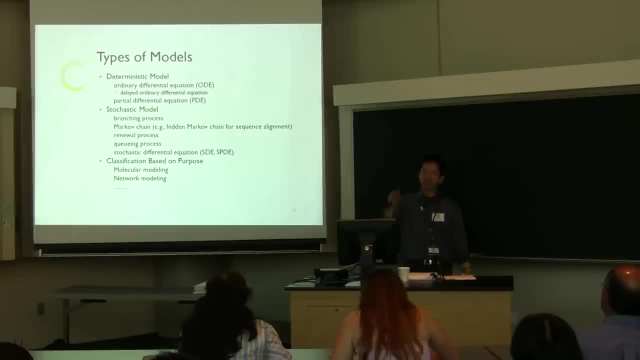 And by this bank you only have three people can serve you And then you have to wait in line And if you're interested in what's the area to time to get served, that would be a queuing model. So this one is the classical differential equation. 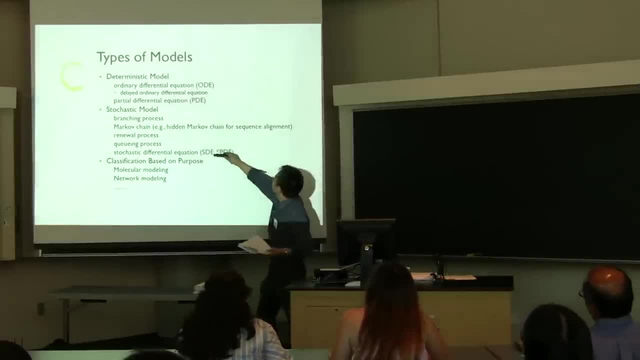 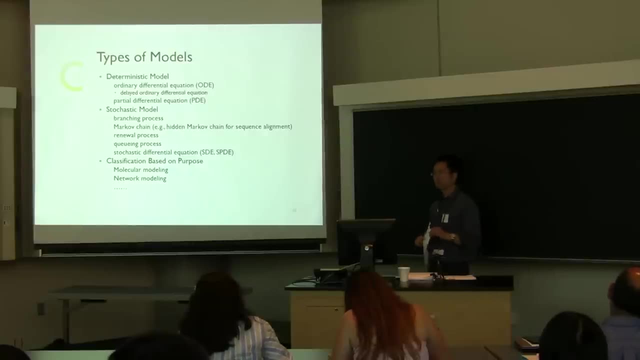 which means we introduce randomness into ODE or into PDE- OK. So good thing that now we extend ODE- PDE to model randomness- OK. The bad thing is that whatever problems ODE, PDE have, OK, the SPDE also have OK. 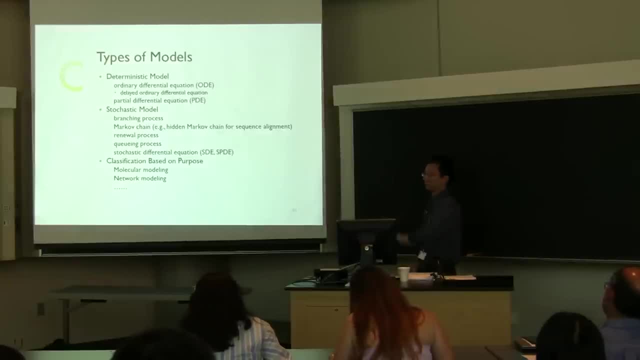 And they have actually more problems than ODE PDE's for talking about how to use this model to interpret data. OK, So, by the way, it's just probably take it as a personal opinion, OK. So the last one is: you can also actually classify models. 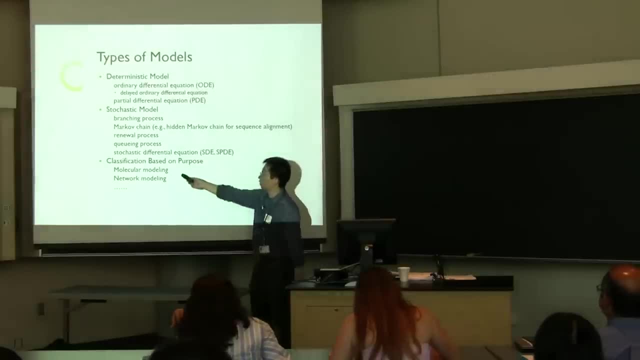 based on your purpose. OK. For example, if I want to do this, if I want to do a molecular modeling, I can just use the molecular dynamics. I can also use quantum mechanics, right, if I really want the accuracy. OK. 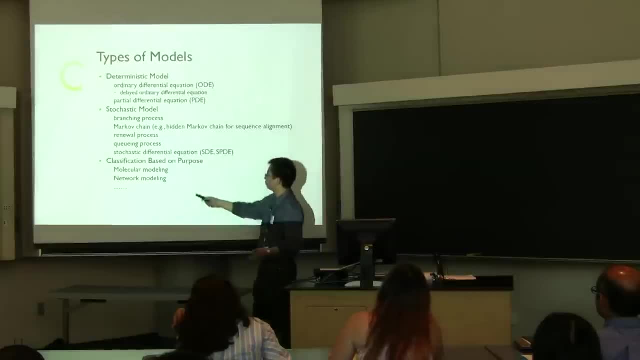 Also I can use different models to do network modeling. For example you can use the Boolean network, Bayesian network, model, ODE. Also, of course, you can use ODE to model network. So it depends on purpose. You can also use different types of models. 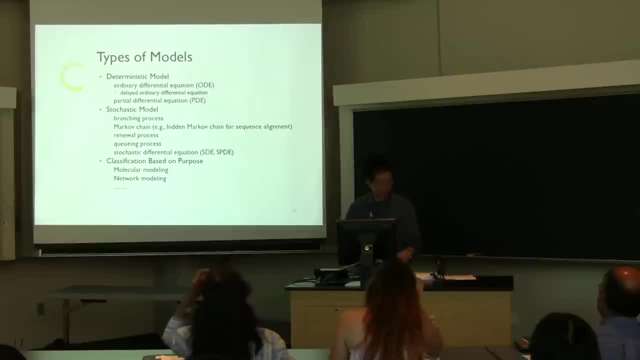 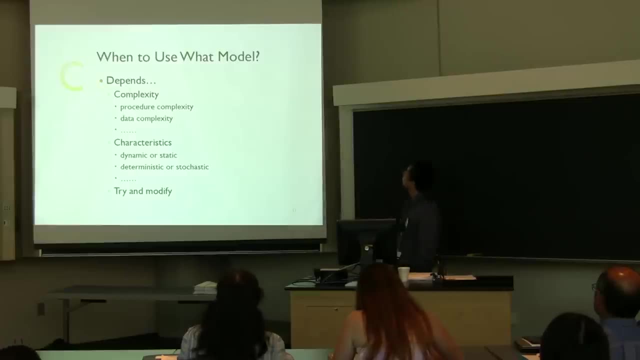 So that would be too much to actually go through. OK, Now let's talk about when to use WACC model. And the answer is actually disappointing because I probably give you too much hope. OK, at the beginning of this talk, 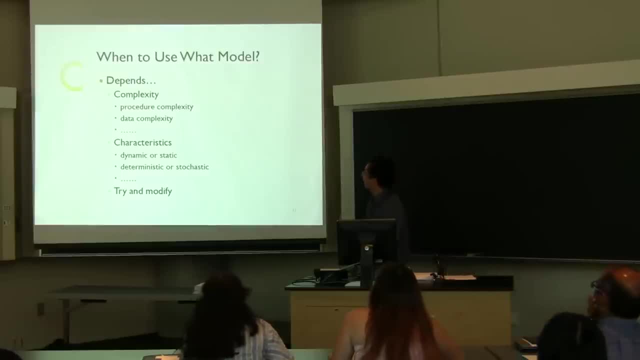 But the answer actually depends Depends on what Complexity the first one is: You don't want to use a very complicated model to model a simple problem, And also you don't want to use a very simple model to model a complicated problem, right? 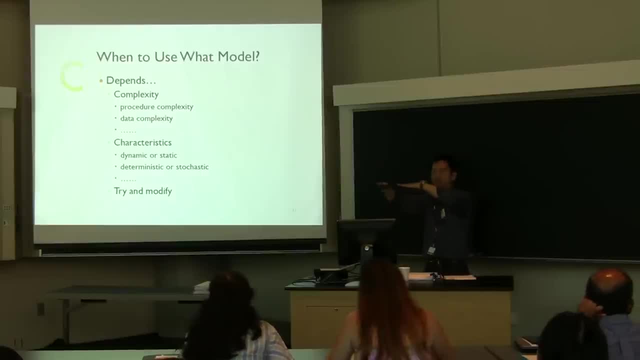 You have to match the complexity, OK, between the model and the real problem. So the complexity can come from the procedure. It can also come from data. So procedure, for example, if we want to understand the key cell activation, OK. 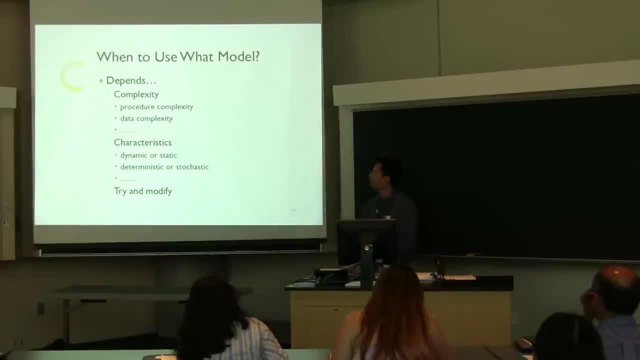 you know, there is tons of steps involved and many factors involved. If you want to create a model for that kind of thing, OK, you do need a complex model. However, sometimes the problem may not be that difficult, but data is. 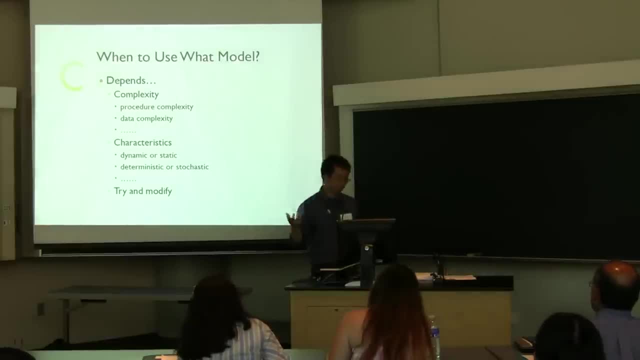 For example, if you want to understand the study that you know, HIV dynamics in patients, OK, the model we usually use actually only have three variables. OK, So three variables, three equations. However, we're going to collect data from hundreds of 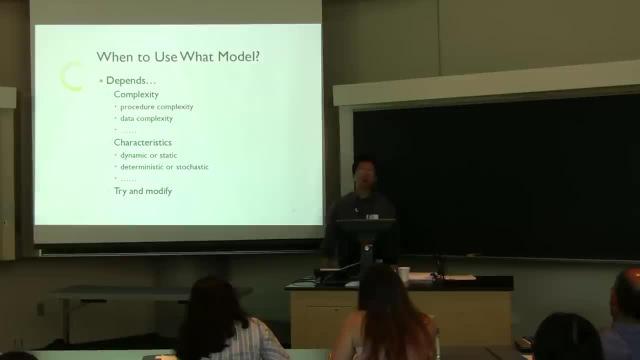 sometimes it's thousands of patients. So how to infer, OK, the kinetics parameter from a population of subjects? This time you have a complicated data set. So, in that sense, you want to have a complex data set. So, in that sense, you want to have a complex data set. 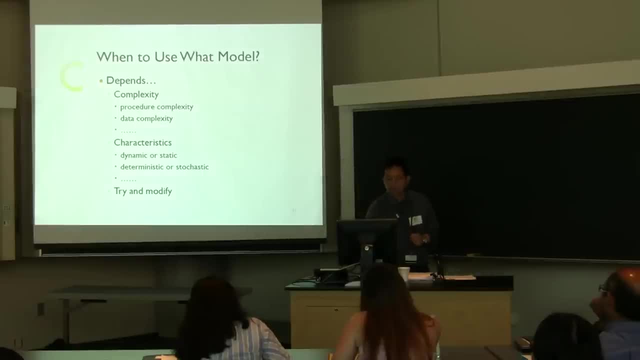 You also have to consider, OK, data complexity. Actually, on Tuesday, that's where I'm going to talk about one example about this data complexity. OK, That's called actually mixed effect model, OK, And also you need to consider the characteristics. 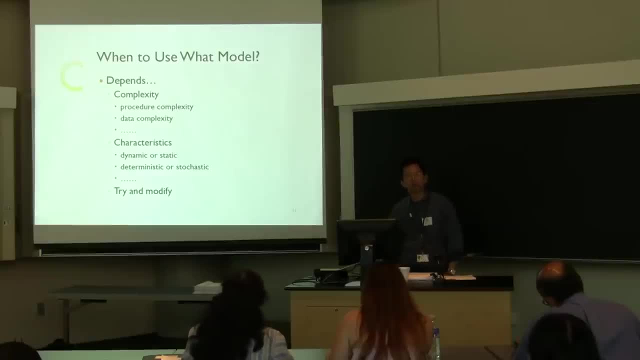 of the problem. For example, if it's a dynamic problem, then you have to use a dynamic model. If it's a static model, a static problem, then you just use a simple static model. So what? I think there is actually a good example, OK. 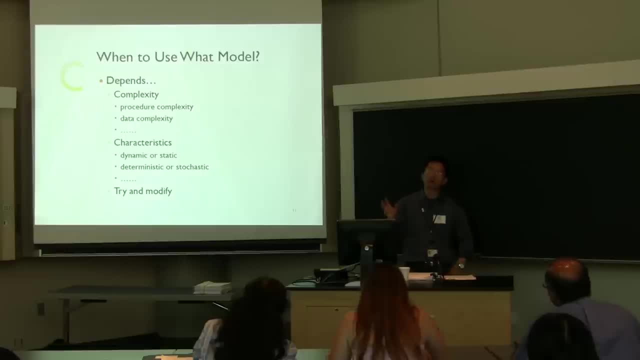 when people do the gene regulatory network modeling. OK, you know that gene expression is actually is a dynamic pattern. OK, It's not static. Doesn't mean that we collect data on day zero and day five and compare them. Then everything is clarified. 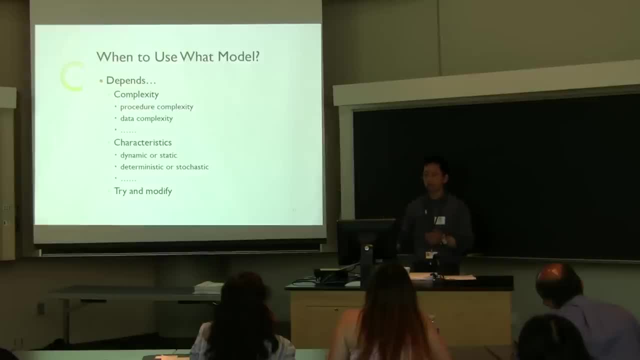 No, it's not that way, Because if you look at the data, OK, you have an upper end data, You have an up and down pattern, So you have to take that time course pattern into consideration when you model that. Anyway, oh, OK, I forgot to mention this. 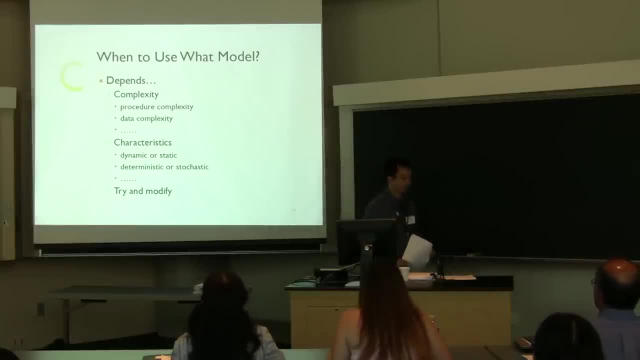 So sometimes you also have to choose whether you want to use the deterministic model or the static model. I leave that to tomorrow. OK, this part. I'm going to show you some example. OK, When? OK, deterministic model is OK. 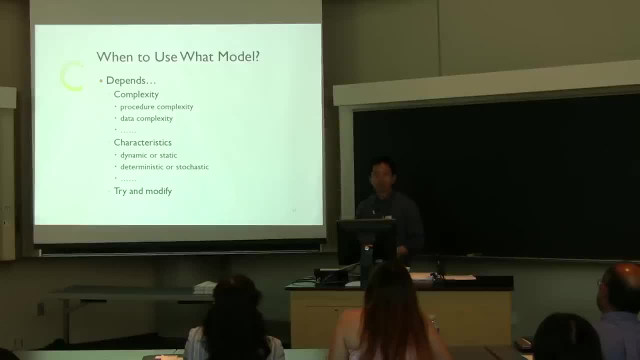 OK, And when you have to switch to static model And eventually, OK, even we do like we do modeling every day, we have to try to modify. OK, whatever you see in the publication, That's probably after you know, a series of modification. 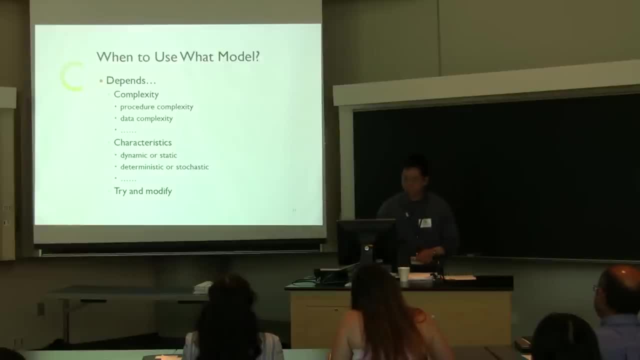 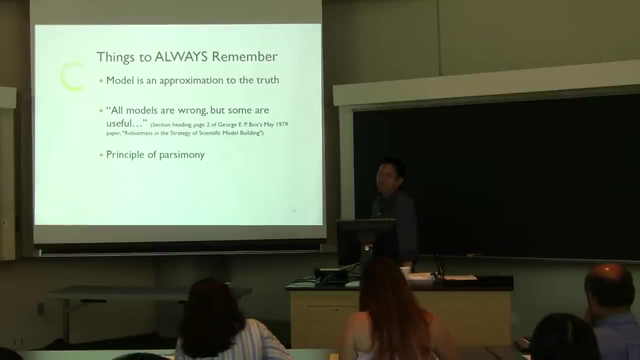 and refinement. So OK, so this is some cliche, OK, I have to mention every time. The first one is: We talked about OK model is approximation to the truth. Second one: you can hear this everywhere, OK, 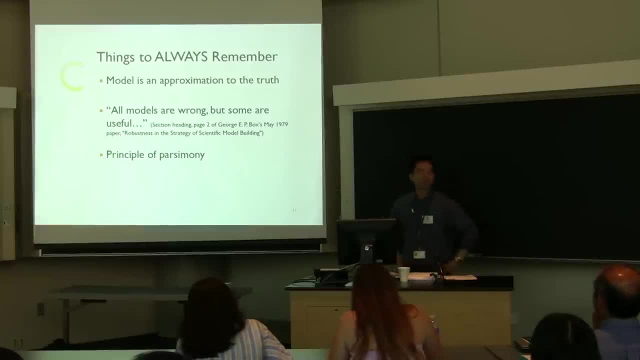 Models are wrong, but some are useful And I particularly figured out a box where it come from. OK, So models are wrong because they are approximation, which doesn't mean they are really wrong. They are wrong because they cannot take all the factors. 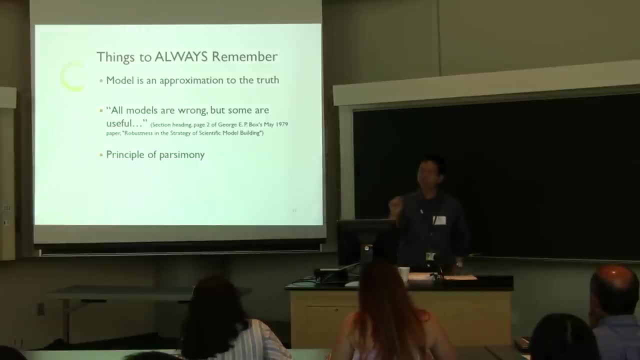 into the model. So if you want to write down every detail, OK, in your model, even for a very simple problem, for example the infection in the lung, you will get hundreds of equations. OK, Use that model. you cannot do anything actually. 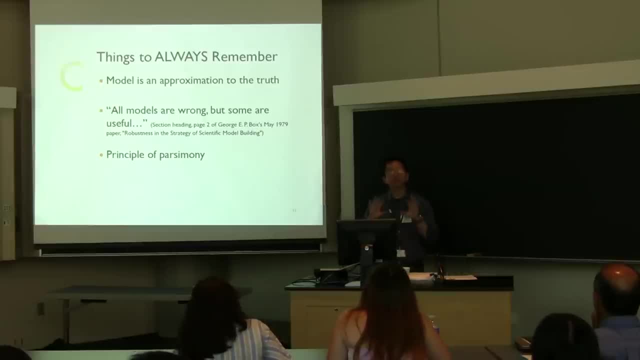 So we actually sacrifice, OK, some unimportant details And we just focused on those factors that we believe they are significant or important. So that's my understanding, OK, why people say models are wrong. However, since we captured them And we captured the main factors of players in this game, 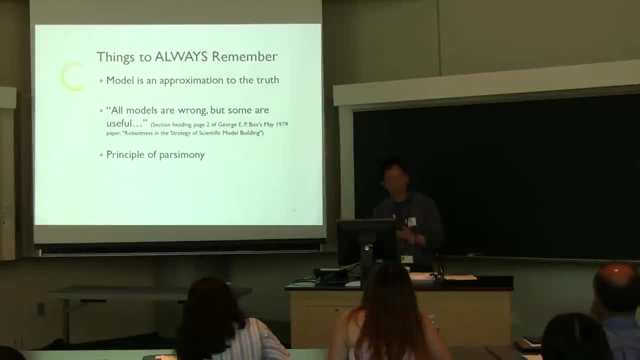 we definitely can use it. OK to interpret something, But to me, OK, I prefer to use the principle of parsimony because, like I said, you can always create a very complex model. OK, as you want, However, to interpret your data, I. 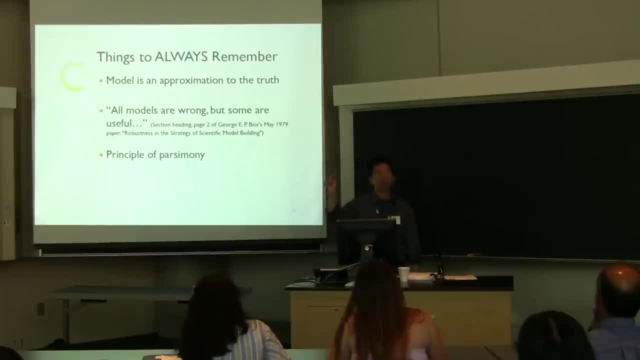 would prefer to use the minimum number of equations or variables or parameters. OK to interpret. OK, OK, OK, OK, OK, OK, OK. So that also related to the identifiability issue that Martin has mentioned From our. we're going to actually talk. 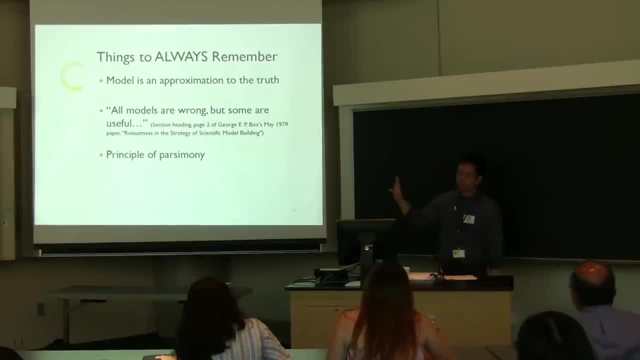 about the identifiability issue. So for now let's just say, OK, if we can use the minimum number of variables parameters to well integrate a problem, then go ahead. do that OK. So I don't bother to intentionally create. 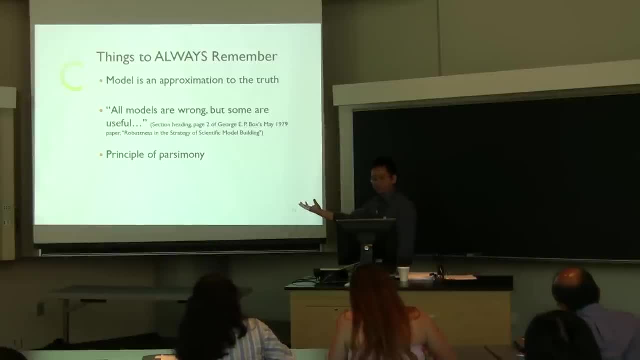 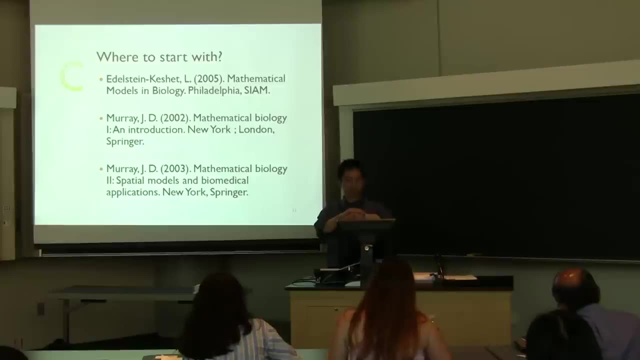 a very complicated model and then to model data. Sometimes I can actually give you trouble, So now I still have like 20 minutes, so let's do some simple math actually, If you're really interested in the mass-based modeling and 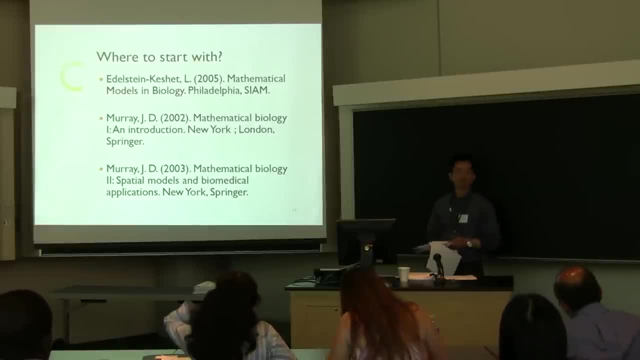 you're not constrained yourself to what we teach here. here are three books You probably can read, And this one. we are from the same person, Marie, And these are good books, but there are some typos. if you can tolerate that, 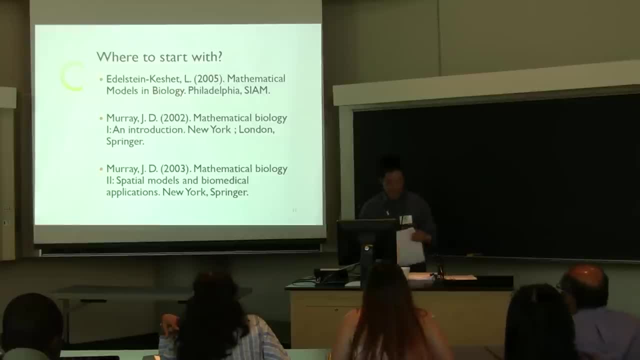 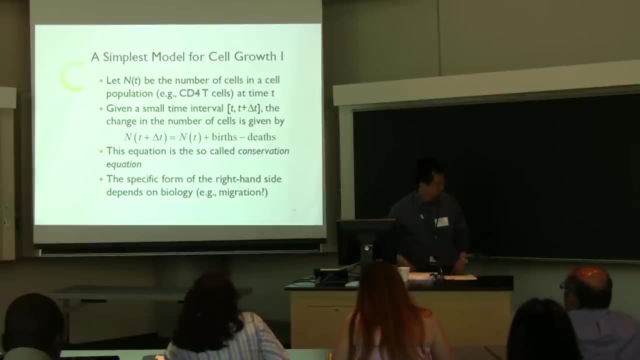 So next one. let's look at the simplest model, for example. Now let's start to talk about numbers. OK, When we talk about numbers, Otherwise they're going to be numbers. So let n be the number of cells in the cell. 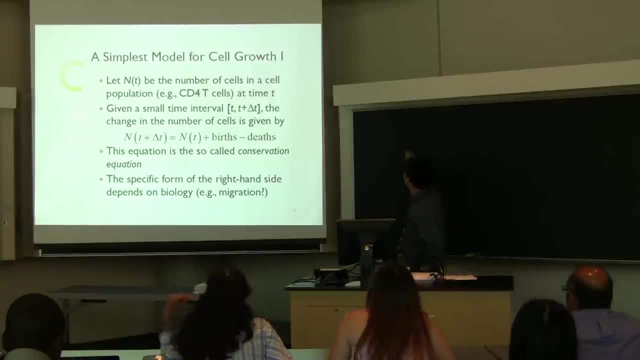 population at time: t So n. here is the number And this one is the function of time. That's the notation. So, even a small time interval from t to t, plus delta, t so n. here is our time interval. OK, We want to look at the change in the number of cells. 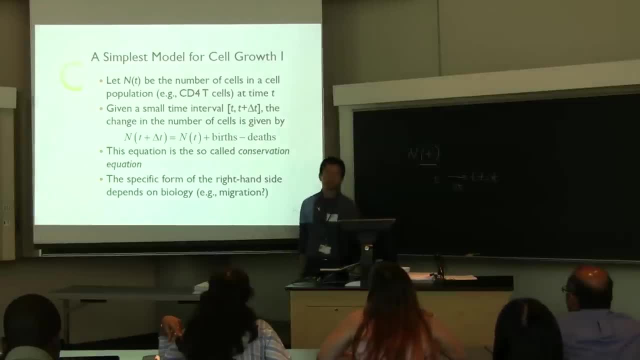 So what mechanism we can actually consider. Of course I can add the number of newborn cells right, And also I can subtract the data cells So they either were born during this delta t or they become dead during this time interval. OK, 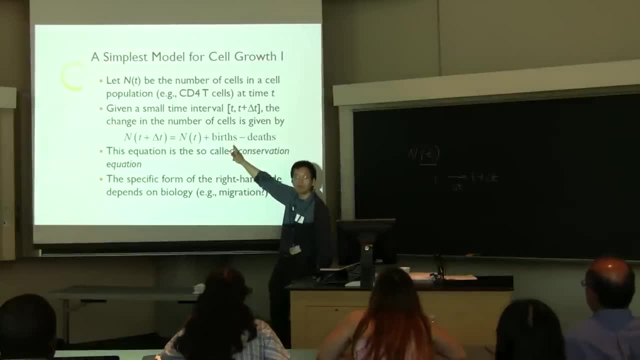 So, although this one is very simple, but we're going to use this again and again and again, especially tomorrow. OK, So the basic idea is that we look at the change in numbers during a time interval. OK, That's the basic idea. 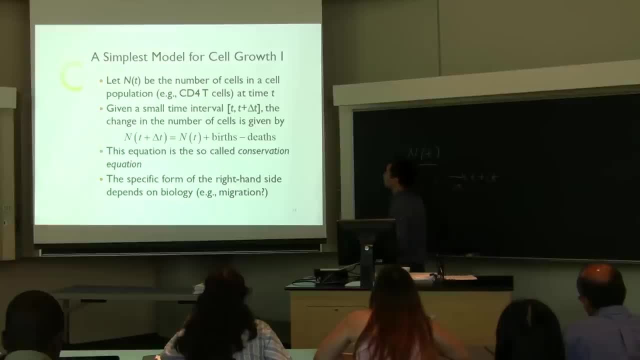 So that's how you actually derive the ODEs. OK, This equation is sometimes also called a conservation equation. It doesn't matter what it does mean. OK, by conservation equation, I don't care, Actually, just sometimes if you meet it. 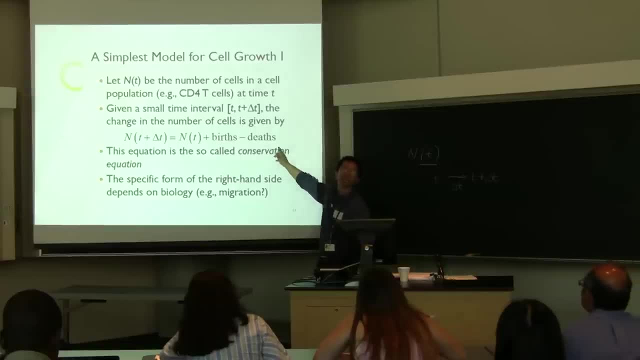 this terminology in a publication or a book? OK, you know what it is. OK, that's all. And the specific form of the right-hand side equation? OK, actually depends on what assumptions or what facts you want to incorporate into the model. 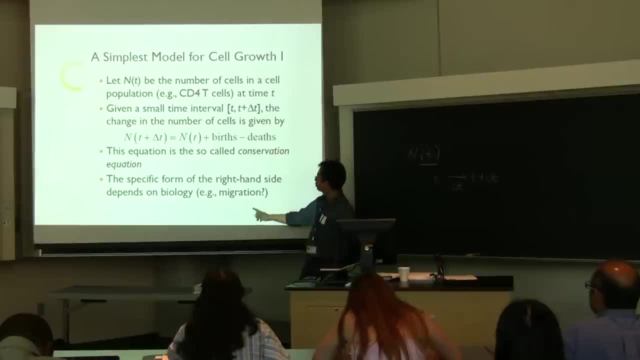 For example, here I only consider the birth and death. If you also want to consider migration, you will have another term. If you also want to consider differentiation, you will have another term. OK, So that's how you start: You start from a simple model and get the one you want. OK. 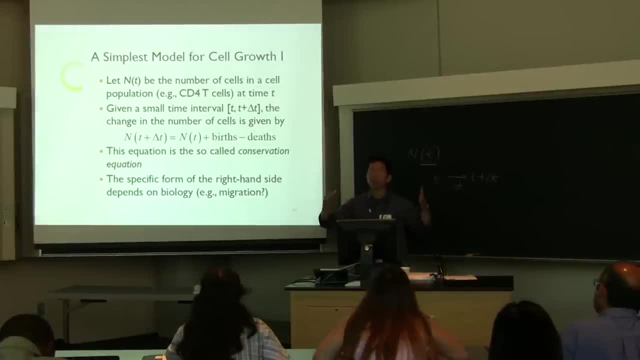 by adding more and more factors you want or you believe that is significant. OK, Excuse me, This conservation equation can be applicable to all biological processes, or you have any restrictions? I don't want to see that because it would be too risky. 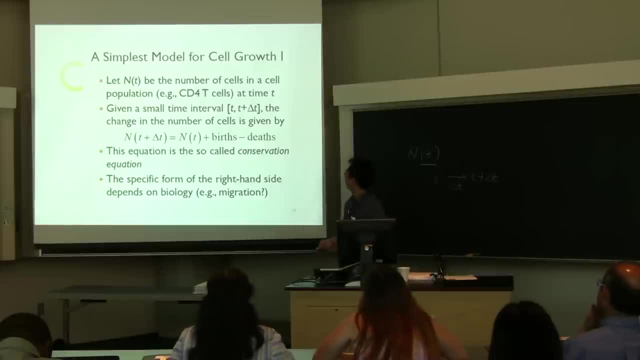 For instance, you said it's a set of proliferation and differentiation. but is it OK If you use ODE? OK, this sort of principle will apply. OK, However, ODE also will fail. OK sometimes, And that's also something I'm going to talk tomorrow. OK, 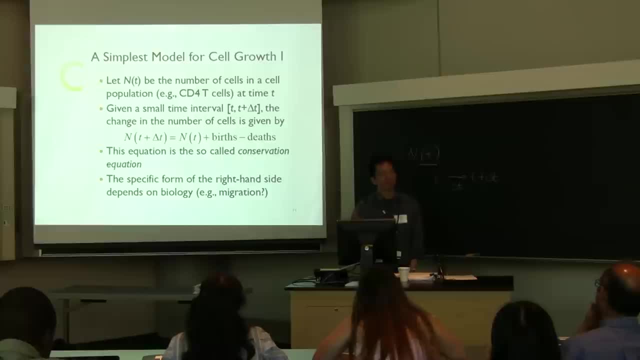 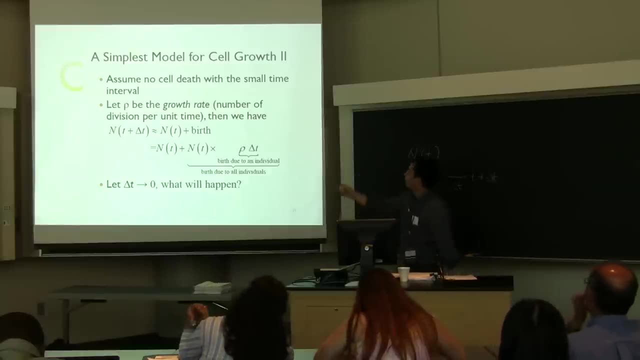 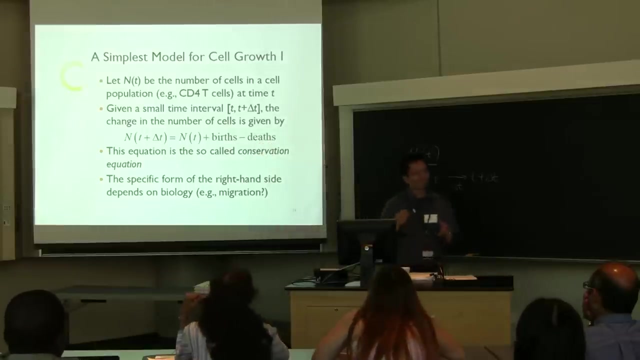 So sometimes you cannot use ODE simply for some reason. OK, So now we already have our first model. OK, That's our first model in text. OK, But let's now turn that text into mathematical expression, OK, So how do we do that? 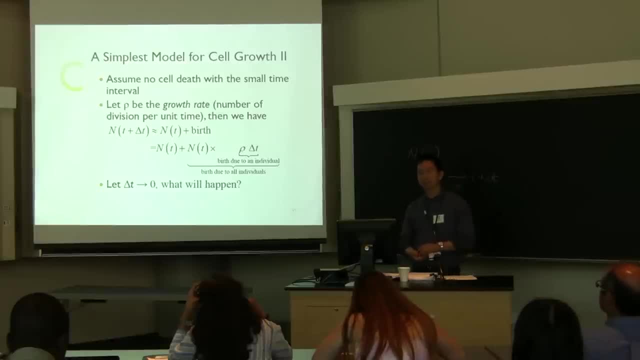 Now it's really simple. OK, Let's assume that there's no cell death within the time interval delta t, So we only consider birth. OK. Now we use rho to be the growth rate. OK, which actually is the number of deviations per unit time. OK, 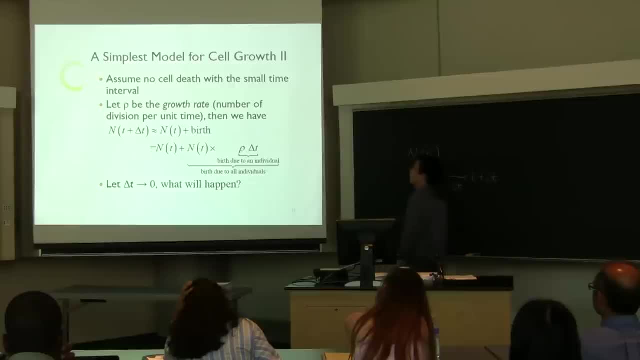 That's the area of rho. OK, the number of deviations per unit time, actually per cell. OK, That's one single cell. The number of one single cell can divide, OK, during the delta t. So unit time, not delta t. 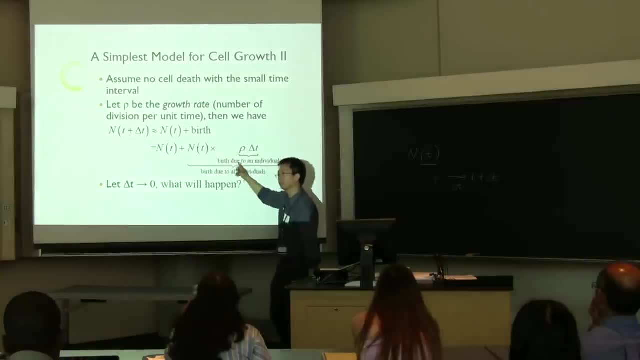 So now let's convert this first to mathematical expression. First, what's the number of deviations for birth during the delta t? OK, That would be rho multiplied by delta t, because rho is the number of deviations for birth per unit time. You multiply the time length, then you 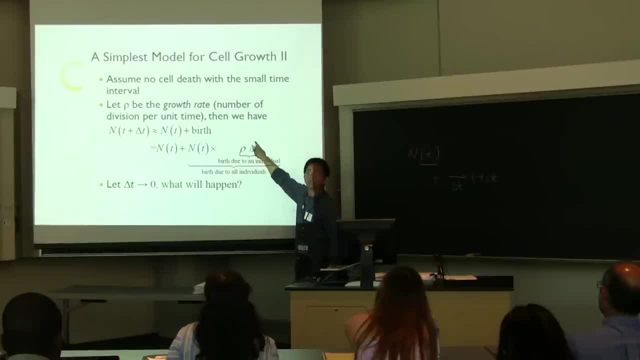 get the number of deviations during this time period. OK, Is that clear? OK, So, however, I come here. We have how many cells we have. We have n. OK, We're not just having one cell. OK, We have n. 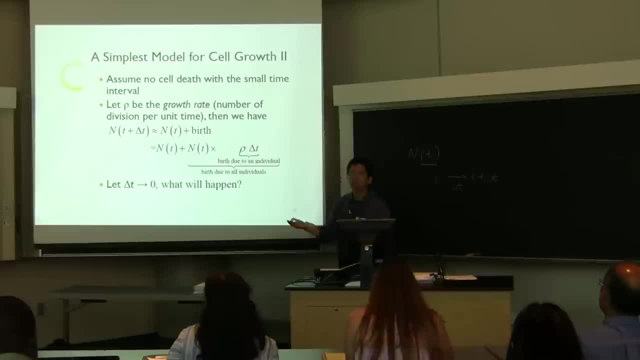 All the cells are capable of proliferate or divide, So that's why I also multiply. OK, N here. Any questions so far? Simple but important. OK, So now I just convert the first term to mathematical equation. OK, What's the next step? 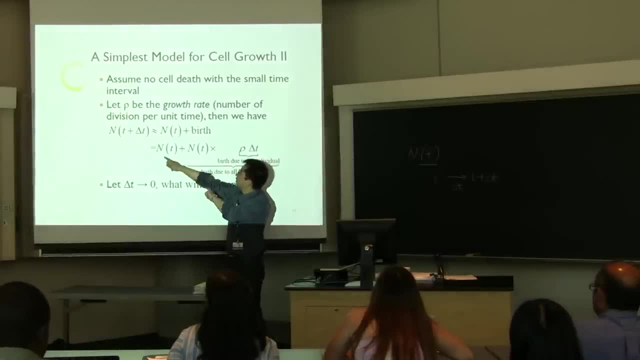 Next step. we cannot stop here, because we know how to predict the number of cells in the population from the number at time t, But we cannot use this equation because it's difficult to use If you want to calculate a number after 100 days. 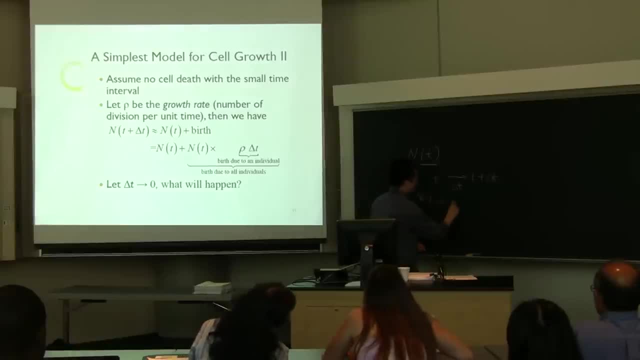 then I have to start from n0. And then I calculate n1, and then I calculate n2.. And here delta is one day right And that would be difficult to use. So what people do, actually mathematicians do? 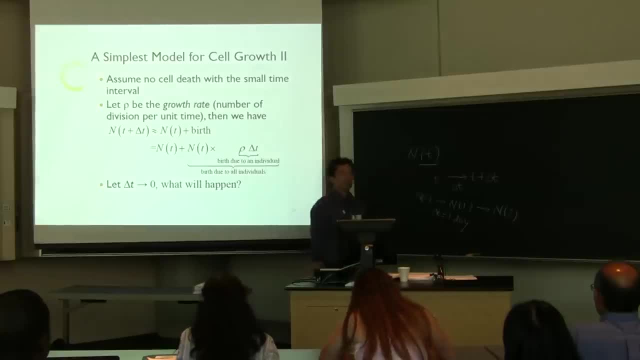 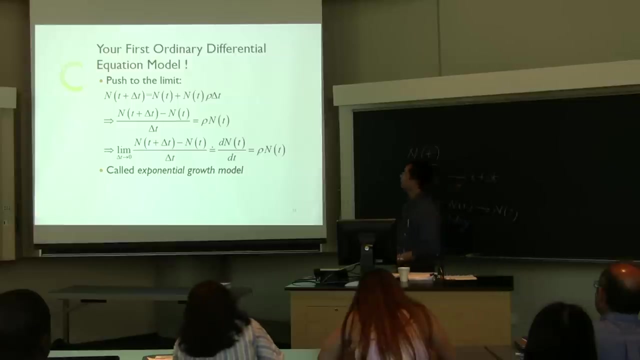 is that we let this time goes to 0. So that sounds unreasonable, right? OK, Because if the time goes to 0, then nothing can happen because the interval is too short. However, if we look at this manipulation, OK, 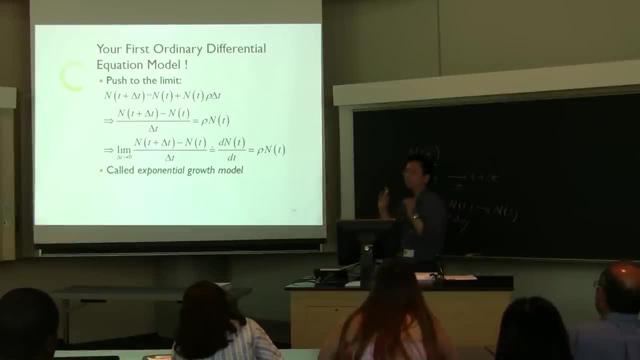 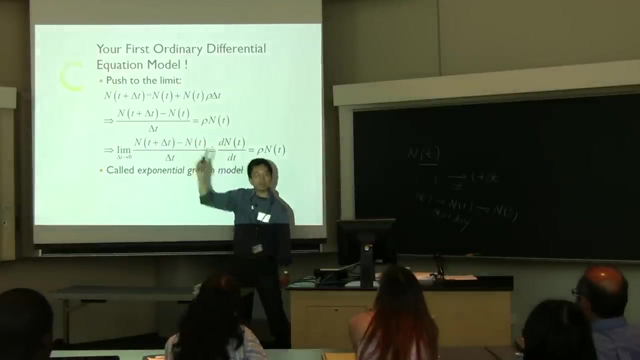 let's call it a manipulation. It actually makes sense. So this is the equation we got right in the previous slide, the first one Now I remove. I move nt to the left-hand side. So from positive becomes negative, You have to subtract, OK, nt. 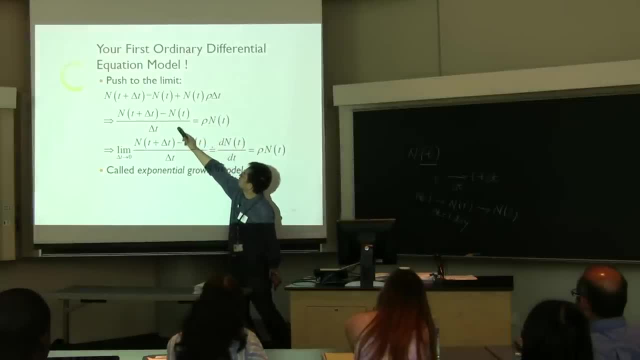 And then I divide delta t out of both sides. So what you get is that the change during delta t is equal to rho multiplied n. So now delta t is done OK from the right-hand side. Delta t only shows up in the left-hand side. 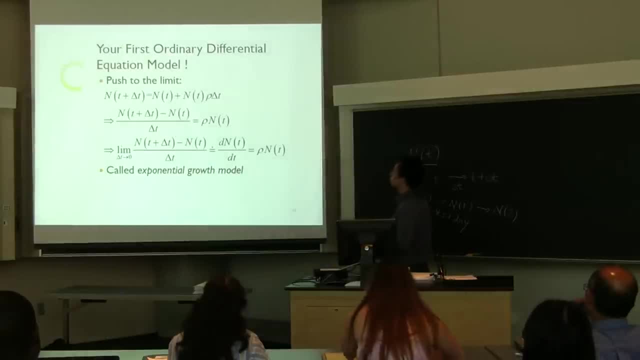 OK. So now, if we let delta t go to 0, what's that? It's something we call the derivative. OK, What is the derivative If we go back to this one? the derivative actually is the change per unit time. 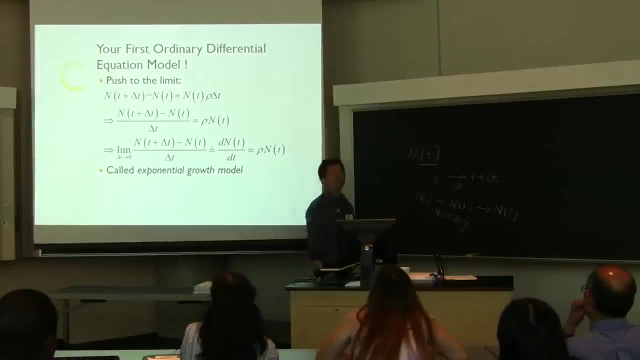 OK. OK, Let's draw it. The change per unit time, that's all the rate, OK, So just for convenience, OK, people use derivative to denote this kind of thing. OK, as d Here d means differentiation, OK. operator. 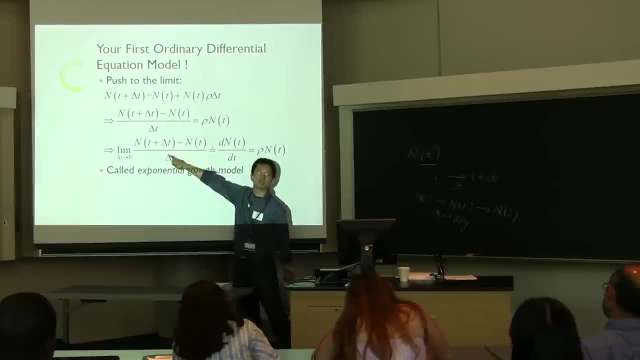 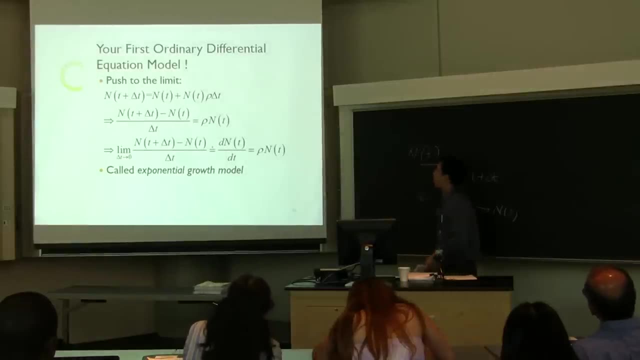 Or you can just remember this. OK, This is the rate, OK, the change per unit time. So in this way we have a, or we want to write it in a different way. So you put a dot here, which also means derivative. 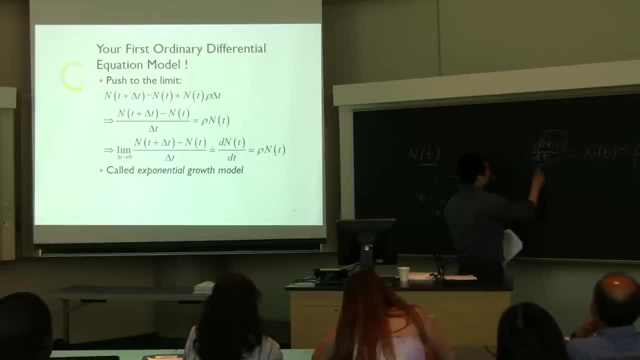 OK, that's the same thing as this one, And sometimes people also write this one, as you can take this part out. OK, And this one means that you take a derivative with respect to time. OK, So you can actually separate them. 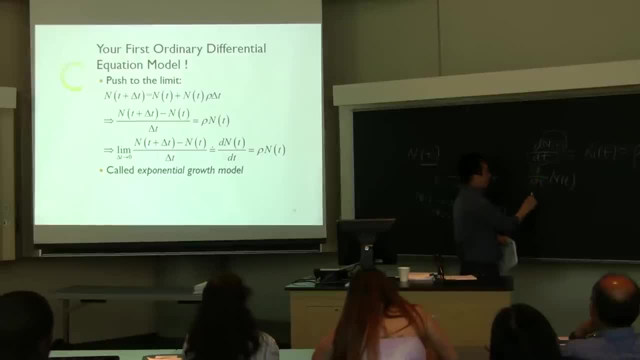 OK, So d here means derivative or differentiation, And n here, which means wherever you want to calculate the derivative, And in the denominator again you have this operator. OK, OK, So d means it's part of the depreciation And the t here is the derivative. 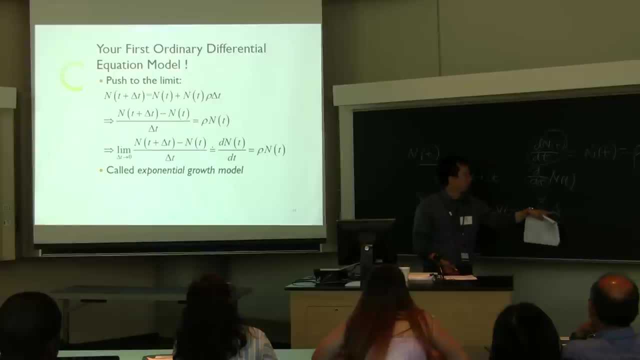 You want to take the derivative with respect to OK, So n with respect to t OK. That's what it means. And for convenience, people also use this notation n dot or n prime. It's the same thing. So they're the same thing, these three things. 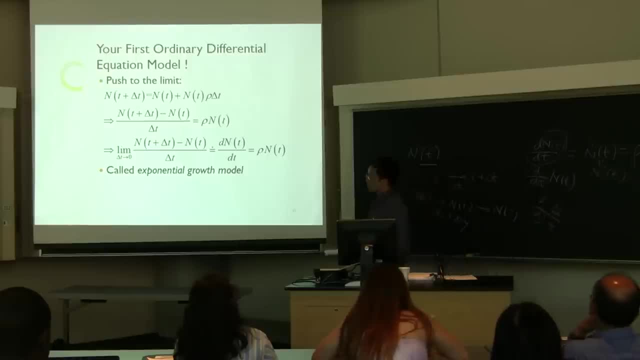 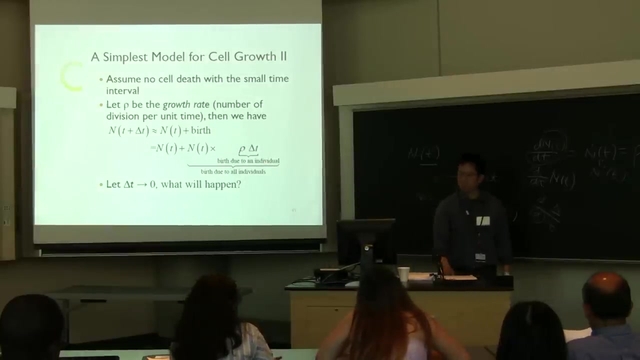 OK. So now, OK, I will be proud of saying we have our first model. OK, series model. and d n d t is equal to rho multiplied n. OK, That's what we derived from here. OK, So this model is also for the exponential growth model. 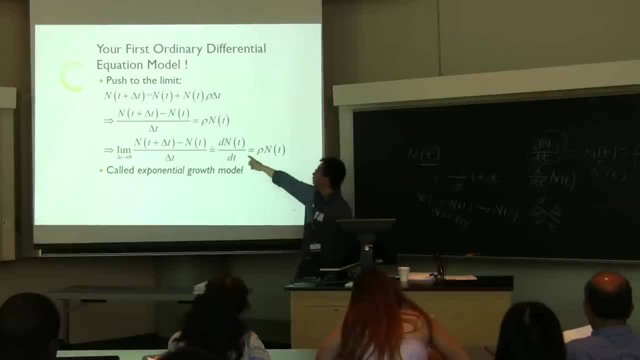 OK, Before I talk about the exponential growth model, I would actually further, I want to talk about this: What's the derivative? OK, So if I draw a path, so we know this number of cells is a function of time, It may look like this: OK, up and down. 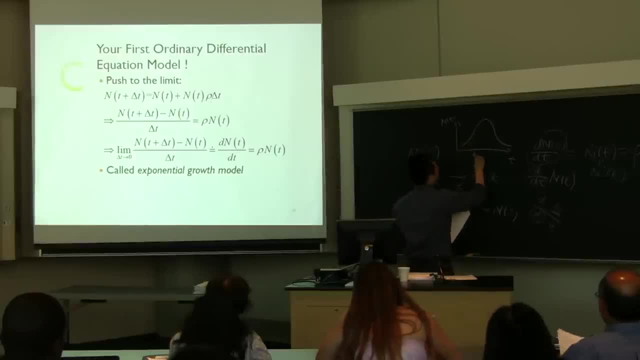 OK. So, given a time point, for example, t 0, OK, what's the derivative here? The derivative here I can use just the slope of the tangent line. OK, Remember, if I have a delta t, OK, that's our commutable t 0 plus delta t. 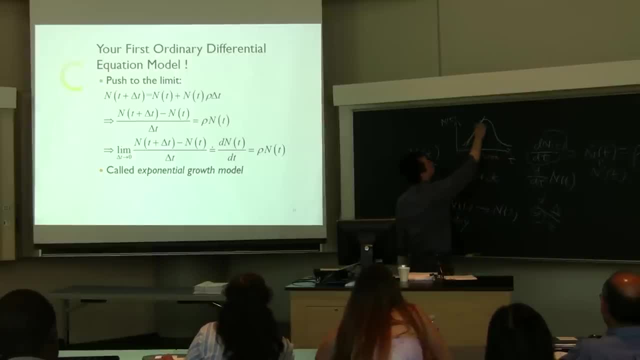 So the length here is delta t And the change in the numbers is here. So you divide this one by this one, you actually get the slope of the tangent line, OK. So the derivative. if you want to understand the derivative using graphics, OK, this will. 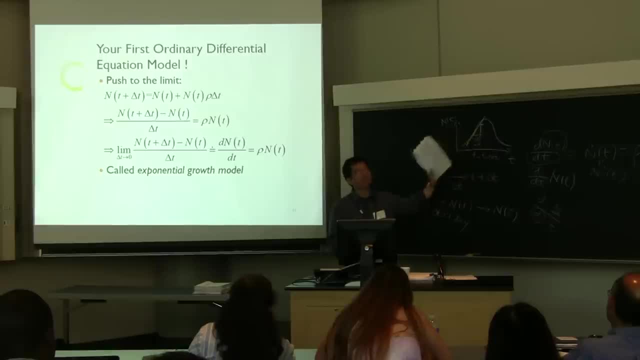 be the graph. OK, The interpretation of: So the slope of the tangent line. OK, That's actually the rate. OK, Again, that's the rate. Right, The change per unit time, That's the rate, Same thing. 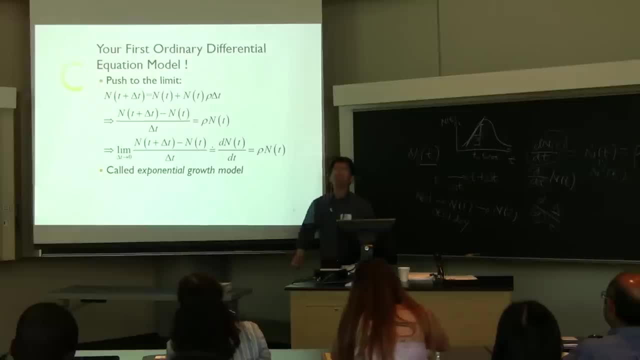 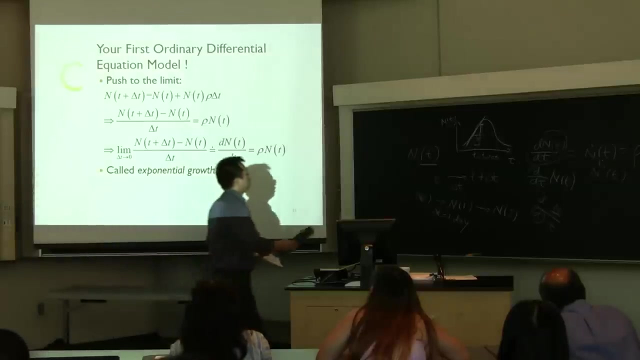 OK, Now let's talk about this so-called exponential growth model. It's called exponential growth model because this model has a close form solution. OK, So not all the models have a close form solution. OK, This is just a very simple model. 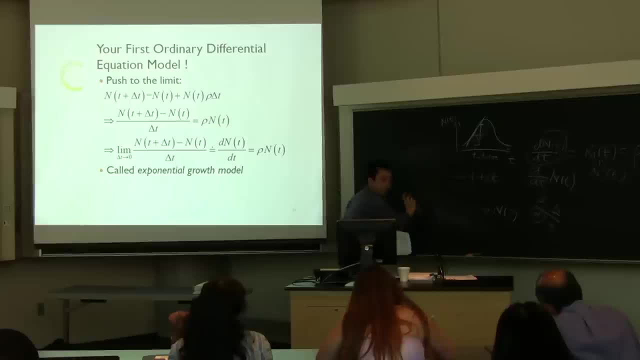 That's why it has a close form solution, And the solution of this model actually is Sir, No, No, Okay. so you see an exponential here, So that's why it's called exponential model. okay, And if you draw the plot, the solution will always look like this way: okay, monotonically. 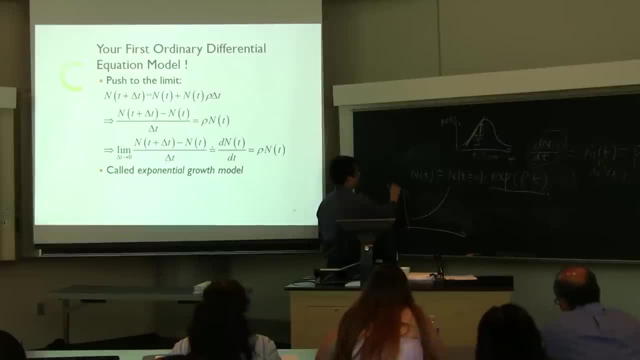 increasing. Okay, the solution doesn't matter what is your initial number of cells in this population, or it doesn't matter, once row is greater than zero. okay, it doesn't matter what's your row. okay, it will look like this: exponentially increasing- okay. 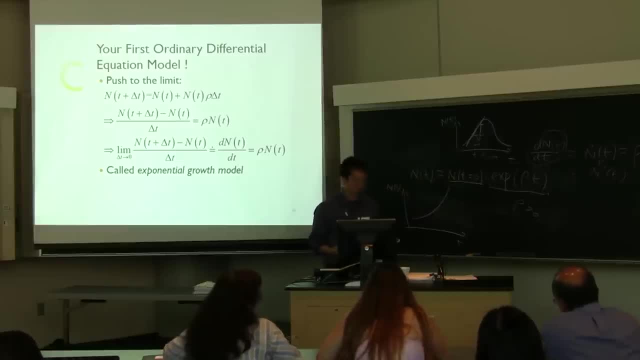 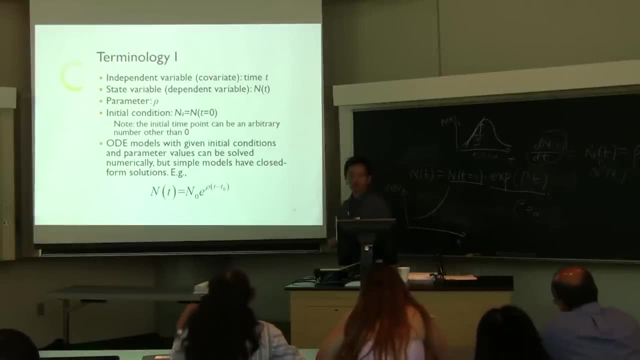 That's why it's called the exponential model. okay, So now, since we have developed our very first model, let's get familiar with the terminology. okay, So you're already. okay, We have, We have something called independent variable in your model. 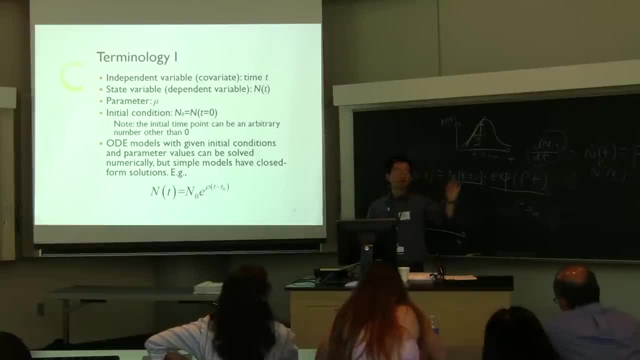 Independent variable means this variable does not depend on anything else, So itself it will explain everything, okay. for example, the time t: okay, We decided to measure the number of cells at day zero, day one, day two. We already fixed that number, okay. 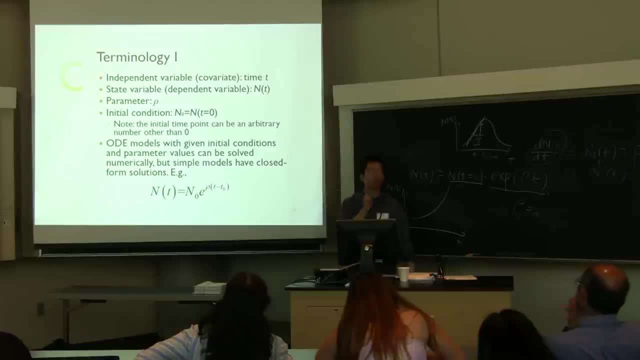 We know everything we are doing. okay, So t itself will not change once we design experiments right, And that's why we call it independent variable. okay, It does not depend on something else, Yeah. however, the number of cells in the population, we call the state variable. 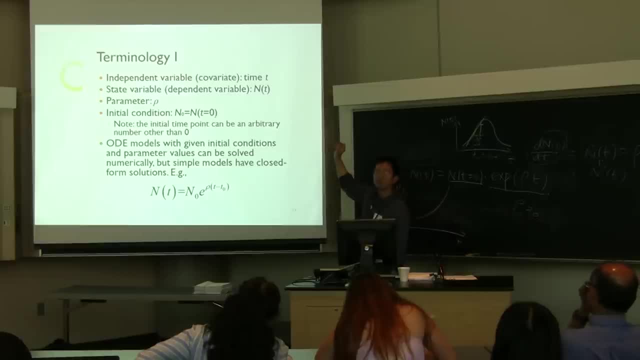 And sometimes we also call the dependent variable, because n is a function of t, which means n depends on t and that is, n will change versus time. okay, So that's why I call it the dependent variable And the role here in our model is called parameter. okay. 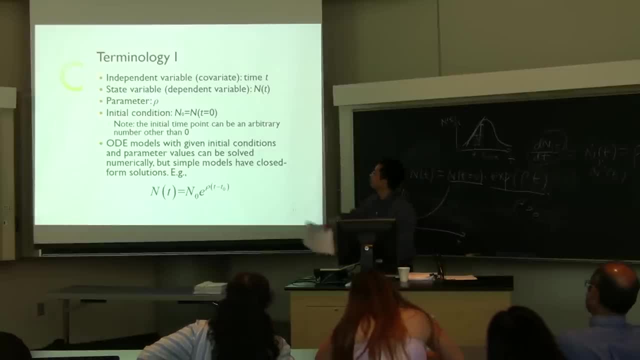 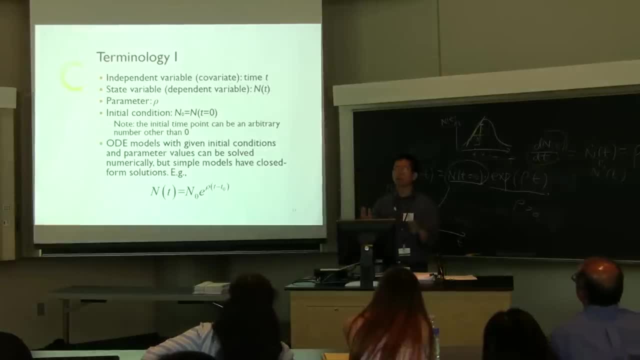 That's a parameter, okay, in the model And initial condition. that's what I wrote down here And also you can see it here. That's just the value of the state variable at time zero. Of course, this time zero doesn't need to be zero, okay. 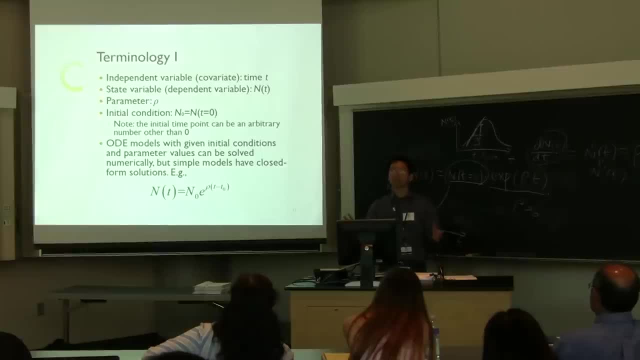 It can be day one, It can be day two, It can be day three. Depends on where you want to start. okay, For example, I do not actually collect data at day zero. Instead, I would like to give it some incubation time. 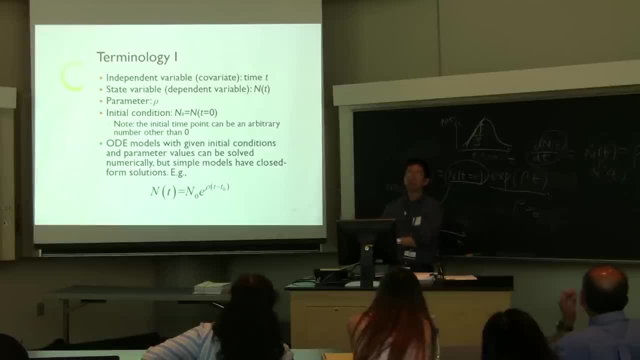 So I start to collect data at day three, Then day three becomes my starting time point And the value of the cells at day three is our initial condition. okay, So I just put zero here for simplicity, okay, That doesn't mean that initial condition should always be zero, okay. 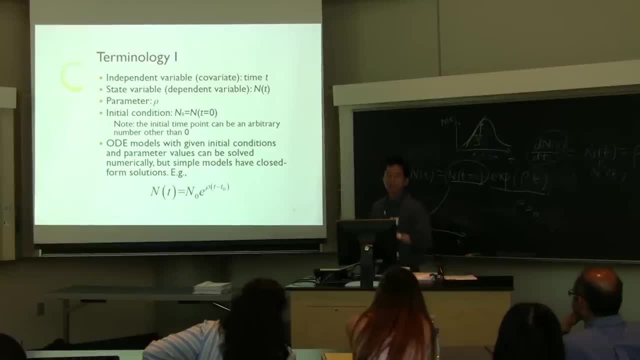 It can be any number. actually It depends on your question. okay, So ODE model: okay, If we give the initial conditions and parameter values, we can solve it. okay. So if I say solve it, which means we can actually get this trajectory, okay, 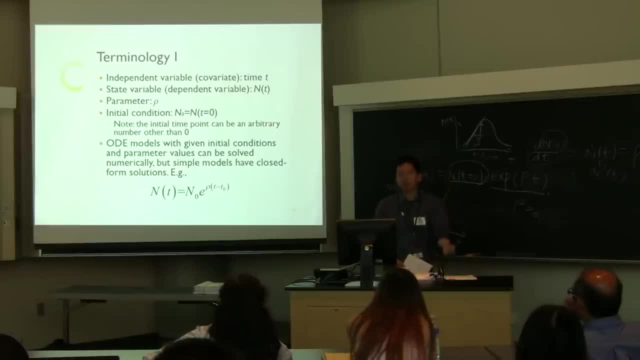 If I have a model, I know the parameter value, I know the initial condition, we can solve it to get this trajectory. So that's the meaning of solving ODE equation. okay, You will know every detail, okay, of this curve. 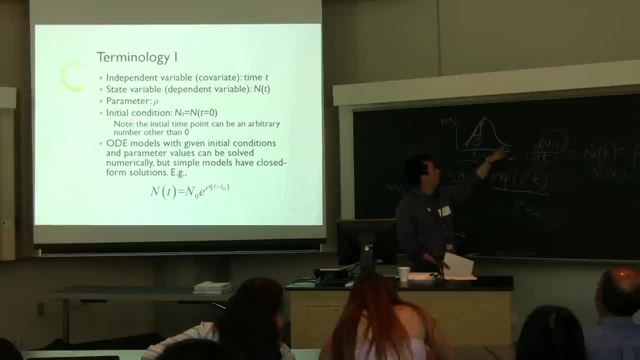 Every point. okay, The value of each point on this line curve, You will know exactly, know the value. okay, That's what it means. okay, So we have talked about this closed form solution. okay, That's the same thing here, okay. 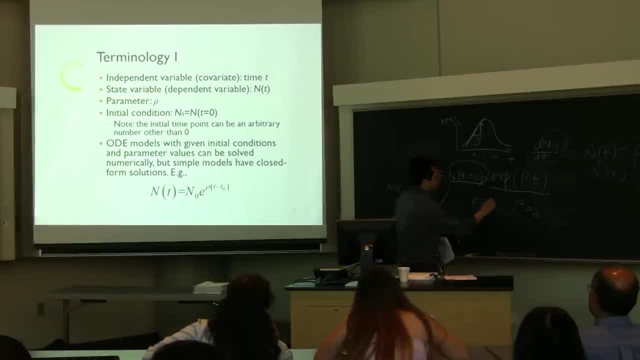 Just, there is some notation difference. okay, You write in this way or you write in this way, They are the same. okay, They are the same thing. okay, So this is a power, you know, to a power of root here, okay. 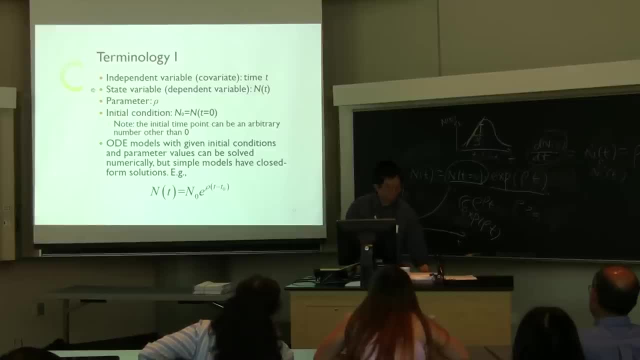 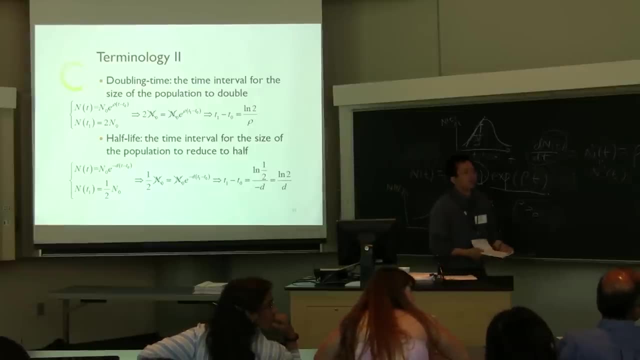 It's the same thing. So questions: so far: No Good. Sorry, With row. the parameters are something that you experimented exactly or there is a concept that you Here? parameter is more like a concept. so far okay, Which means we want to use some symbol to denote the growth rate. 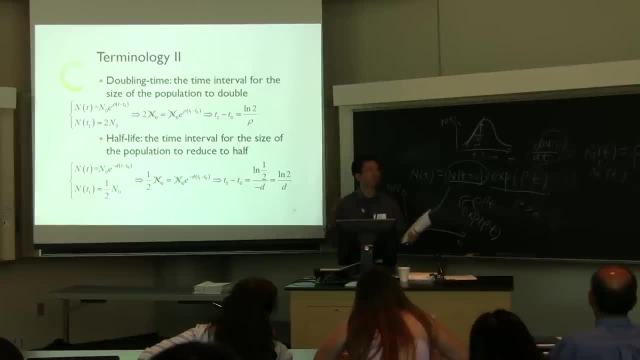 Okay, We know there is something called growth rate in your model And we know that is a row. However, the value can, of course, change If we are looking at the T cells, and this value will be different from the value of. 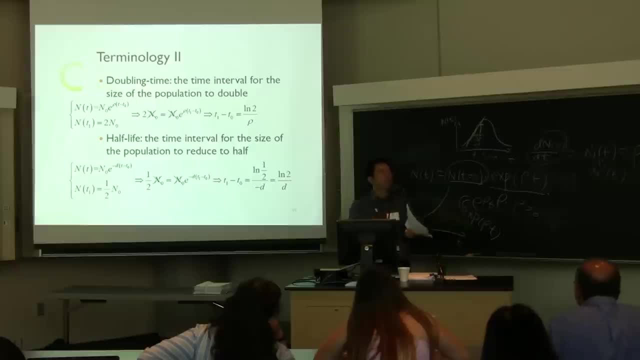 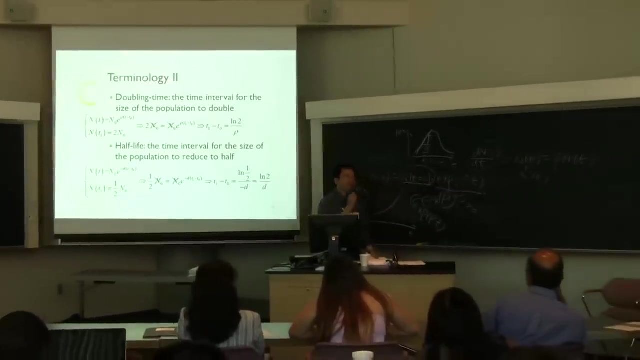 B cells, right. And even for T cells under different stimulation, okay, this row will also change, right. For example, if you change the concentration of the cytokine, okay, the growth rate will change. So you have to plug in a specific value, one specific value, to get one corresponding. 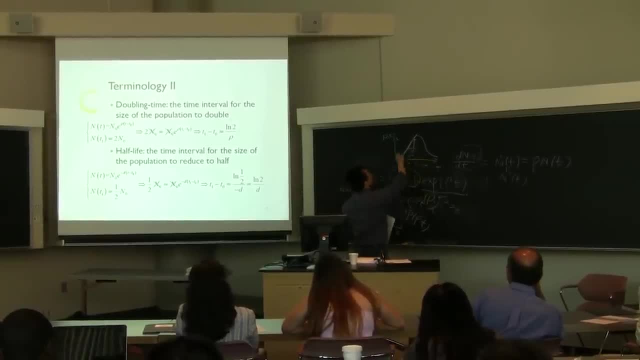 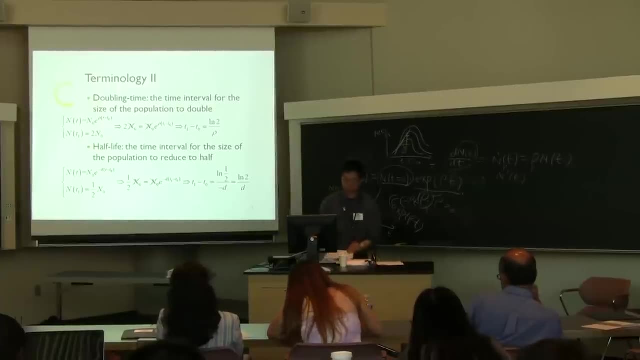 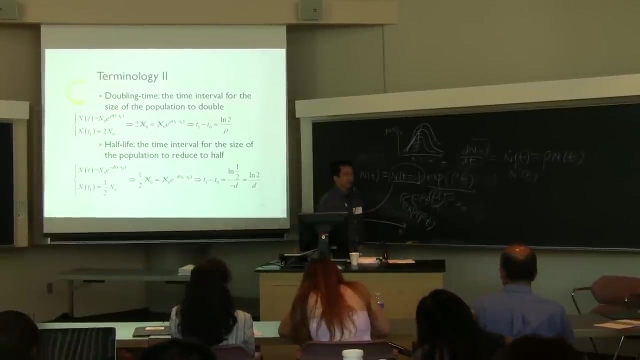 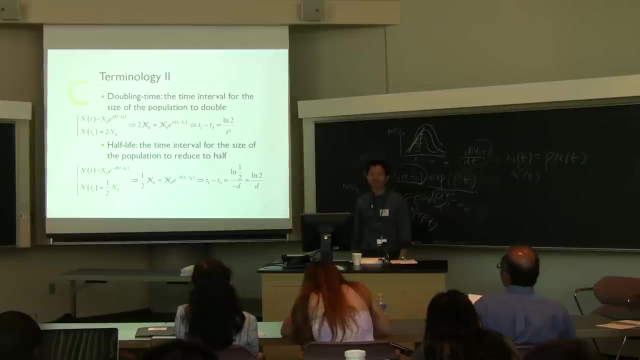 curve And if you change this value, this curve will also change. Okay, Does it make sense? Okay, So now here is some more okay terminology. I believe that it should. It should. I really made this kind of you know terminology before right. 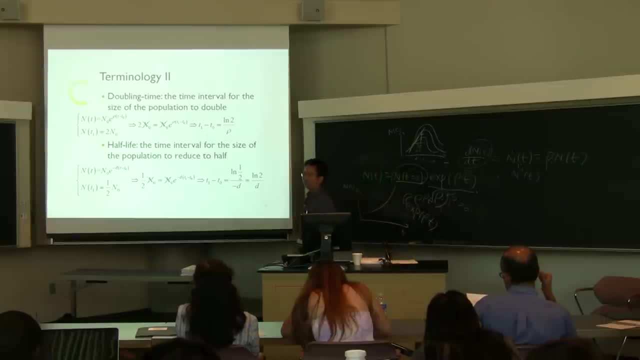 Doubling time, half-life, Okay. So when, When we published the, When Muller published papers- okay, for many times we talked about half-life doubling time. So what does it mean? Okay, So doubling time is the time interval for the size of a population to double. 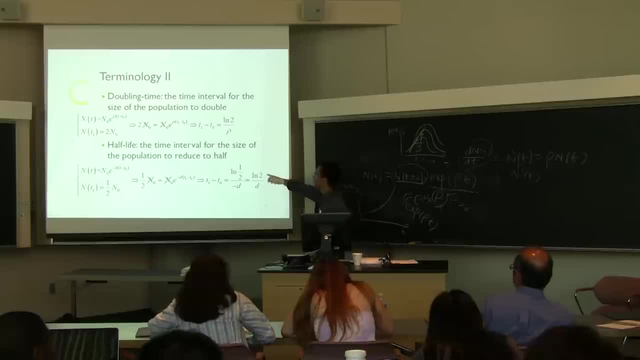 Okay, That's just the Okay. So the definition is simple. Half-life is the time interval for the size of a population to reduce to half. However, In mathematics- okay, the interpretation actually comes from these two sets of equations. 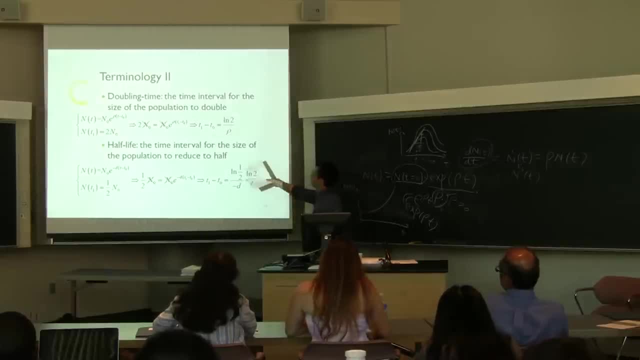 Okay, The first one is that we consider an exponential growth model. Okay, Remember, we consider an exponential growth model. There is something called a linear growth model. Okay, Later we're going to talk about it, So you're going to be different from this one. 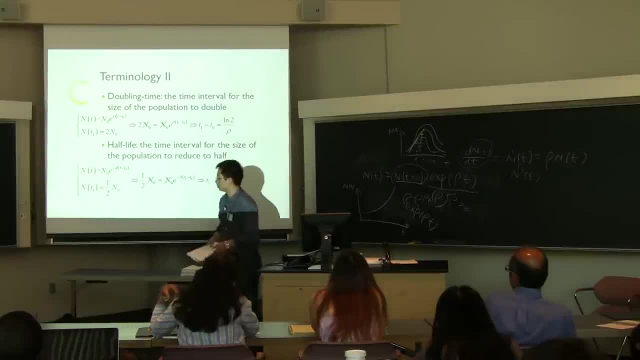 So if we use an exponential growth model, we know the solution. We know the solution, Okay. So the solution is this: one Right, Close-form solution, Okay. So now we want to, After some time interval. now, I let t0 be the starting point. 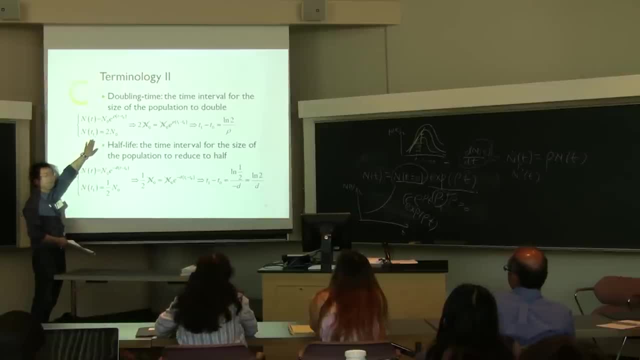 Okay, And after a certain time, point t1, the size doubled. It becomes 2 multiplied n0.. n0 is our initial size of population. Okay, Now it doubled. So after some calculation you can just plug in, okay, the solution into the left-hand. 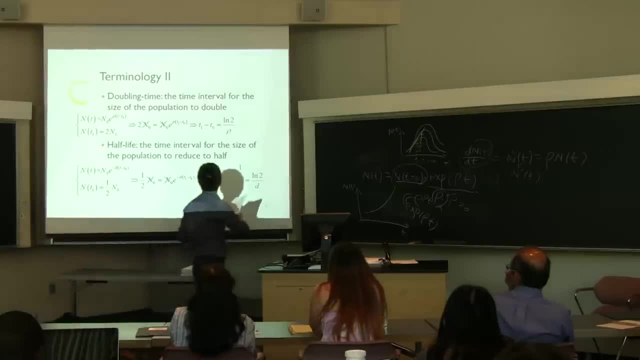 side. That's what you get here. Okay, Plug in the solution to the left-hand side. That's what you get here, And the 2 and 0 just come from here. Okay, Now you cancel out the n0, because both sides have a n0.. 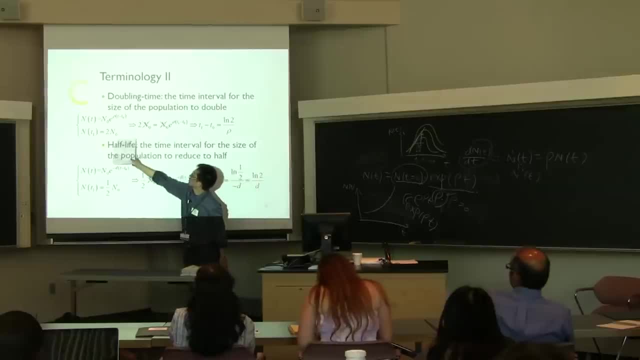 And what's left actually is this one, And eventually you will find that time interval you need. that's the difference between t1 and t0, actually is equal to log 2 divided by rho. Okay, So that's what you get. 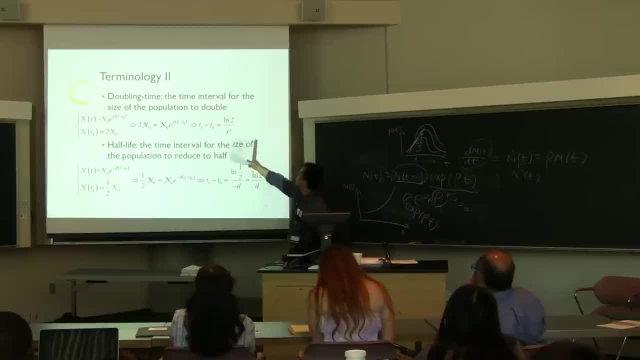 Okay, So that's doubling time. That's how you calculate doubling time. Okay, Once you know the growth rate. so if you want to calculate doubling time, what you do is divide. just divide rho. okay, log 2 divided by rho. 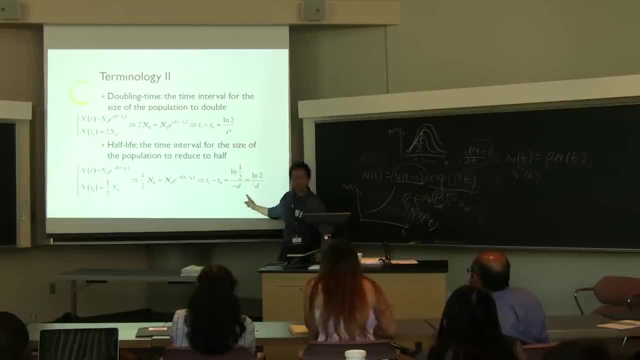 Okay, So to double that. Similarly, if you use exponential death model- okay. instead of growth model, the difference here is that you have a negative sign. Okay, This is death, It's not growth. So the exponential death model will look like this one: 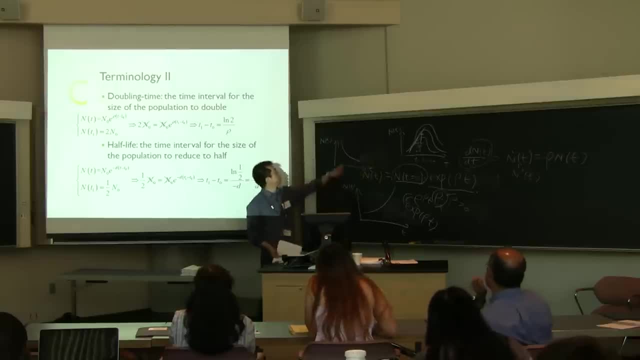 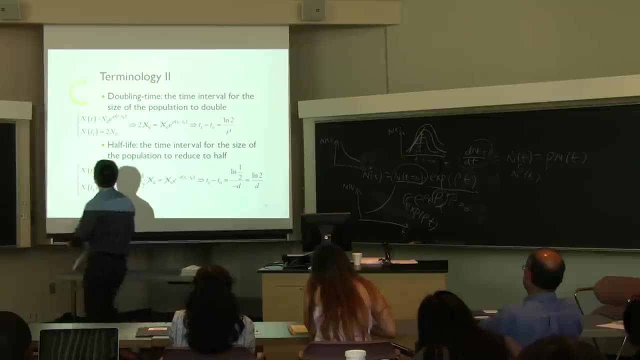 So it will be monotonically decreasing, okay, instead of increasing, because we're talking about death. So the only difference actually is that sign change, okay, between the growth and death model. Now I do the same thing to this equation and eventually we find that surprisingly. 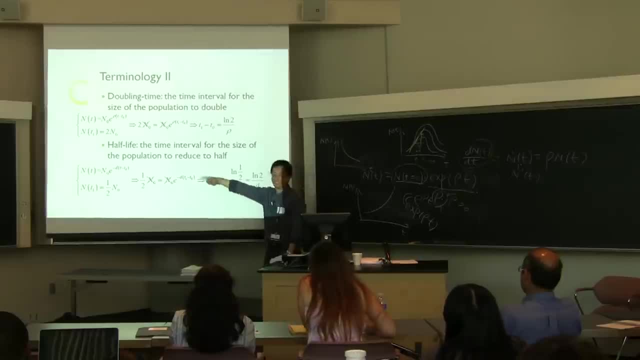 okay, not surprisingly, actually, because the equation is the same, Because the equations are too similar. How do you find it to reduce the size of the population to half? Actually, it's log 2 divided by t. Okay, That's what's called half-life. 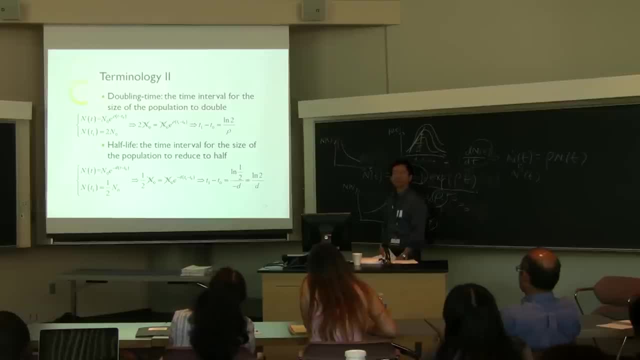 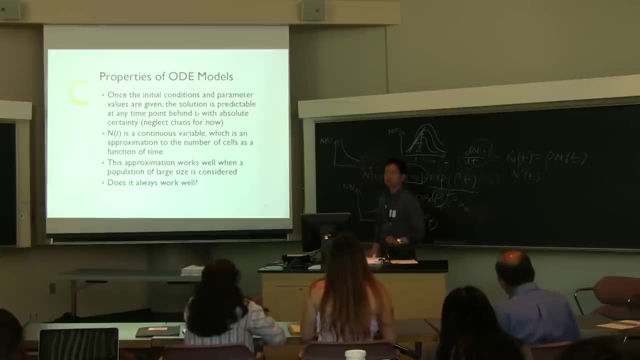 Okay, Question No Good, So I probably are talking to very smart. you know class of students, right, So That actually makes me happy. Okay, So now let's talk about the properties of the ODE models. 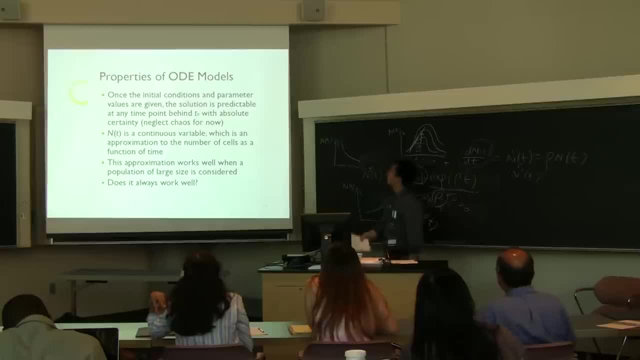 So once again, I want to say that once the initial conditions and the parameter values are given, the solution is predictable at any time point behind t0.. That's our starting time point With absolute certainty. Okay, That's what I just said here. 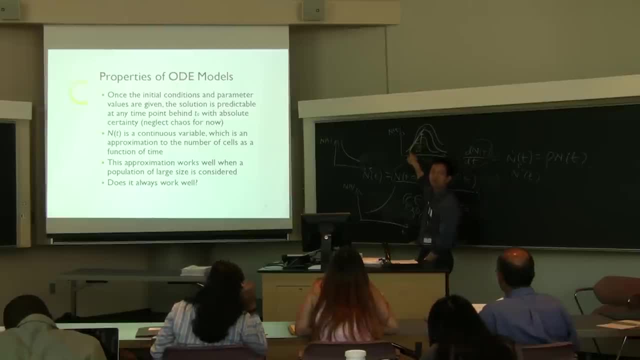 Okay, So if you have one specific parameter value and give it a specific initial condition, then you will have a unique curve. Okay, Remember that curve is unique. Okay, And you can tell every details about one data point on this curve. 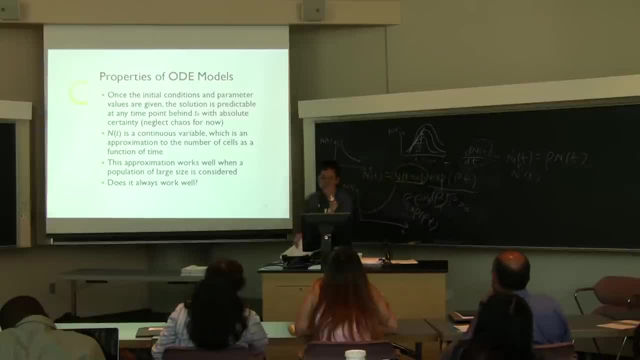 Okay, For example, what's its value? Okay, That's what we care about. So that's why it's called deterministic model. Okay, Again, that's our classification models. Okay, It's a deterministic model. So also we have to note that the NT here is something called a continuous variable. 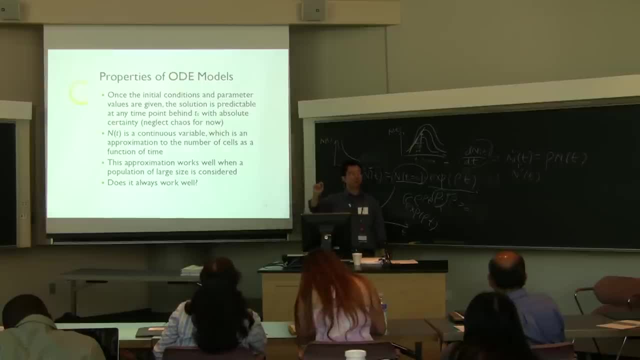 So, although we're modeling the number of cells in a population, okay, NT itself actually here is a continuous variable. So what could be the possible value of cell numbers in a population? 0,, 1,, 2.? 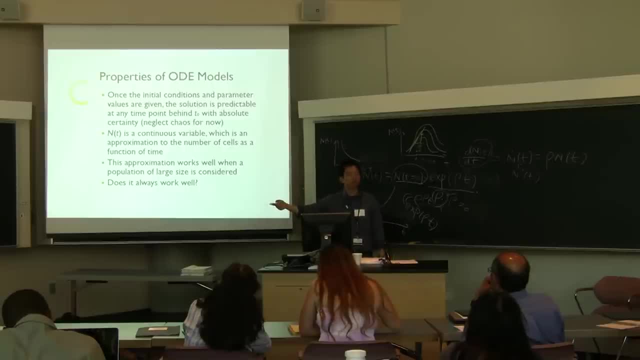 Can you have 1.5 cells? No, Right, It doesn't make sense. However, when we do the modeling, okay, use the ODE model. Okay, NT is a continuous variable, So NT actually can take the value like 1.5.. 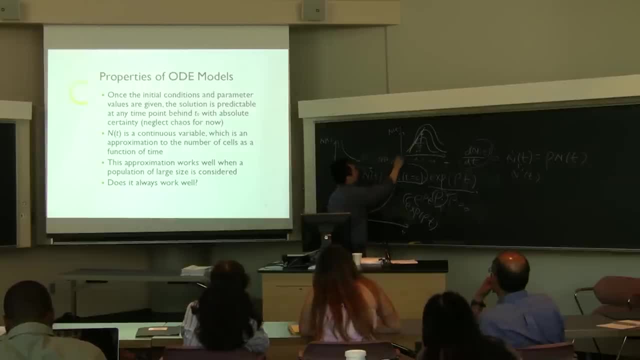 And remember the reason actually behind this is that NT is a mean. okay, What we modeled actually use ODE- is the mean mean number. okay, is not the exact number. okay, You can actually use stochastic model to model the exact number integers. 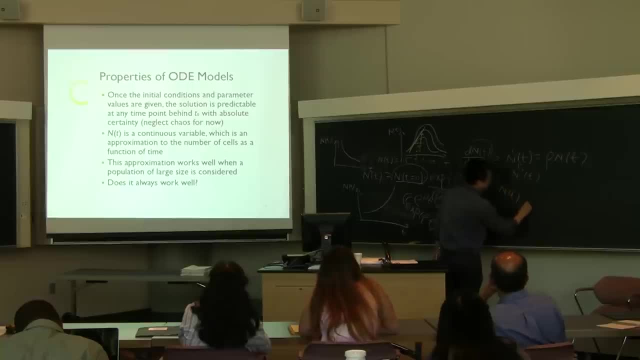 But here the NT actually is a mean is a mean. OK, We know the mean of integers can be a real number, right, 1 plus 2 divided by 2.. The mean of 1 and 2, it's a real number. 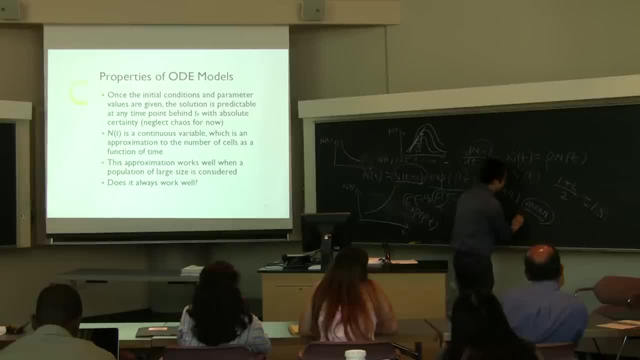 It's not an integer, So that's why, once you use a mean, you actually use a continuous variable. OK, So this approximation actually works well if your size of your population is large. OK, Even if it is a continuous variable. OK. 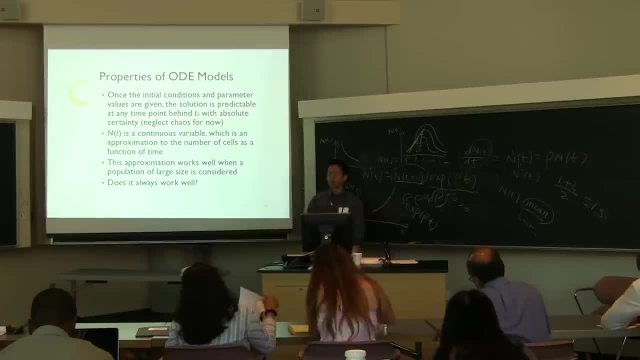 It will work well if your population is large. However, if I say I have only like 5, 10 cells in my culture or whatever, that's time you need to consider a stochastic model. OK, Then you will play with curves like this kind of discrete. 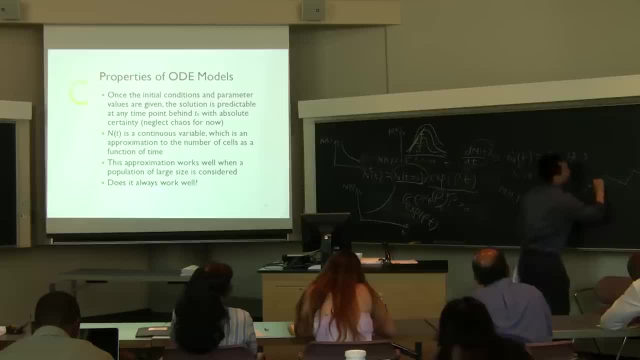 Jump OK, Instead of a continuous curve. So if you use NP, what you get is a continuous smooth curve, And if you use stochastic model, you can now come out with integers, But the results will be like that: stepwise. 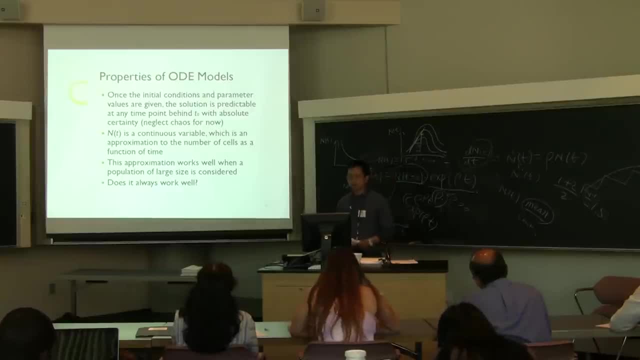 So last question I ask here is: does it always work well, Since I asked it this way, which means the answer is no right, So actually, yeah, tomorrow let's talk about some situations. OK, the ODE will not work well. 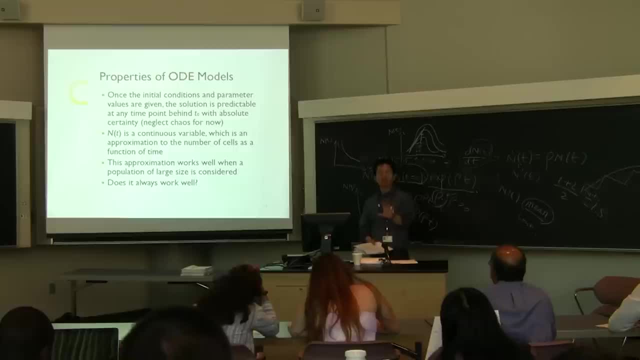 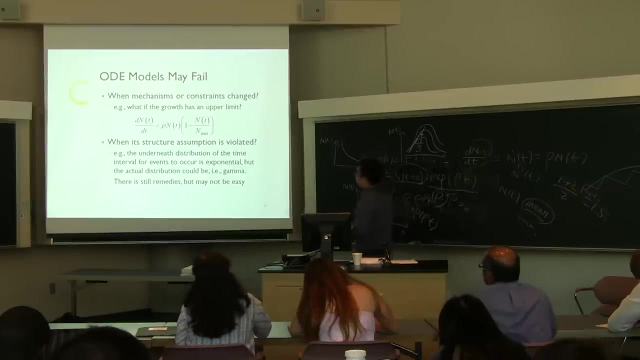 But fortunately OK for most of the cases. OK, in this study you can actually use ODE. OK, But there's just some special cases OK that you have to be careful about. So here I want to talk about the, you know. 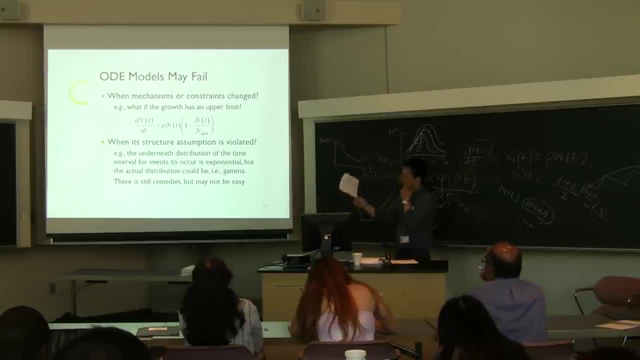 the linear distribution And how we actually make the ODE model OK work better. The first one is in our previous model OK, we're saying that cell will exponentially grow, grow, increase without any constraint. That's not true, right. 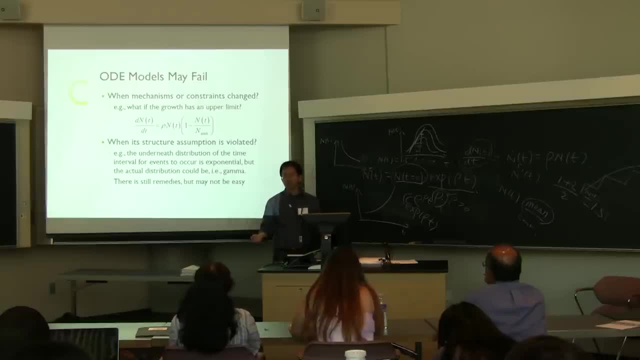 You have limited environmental supply, OK Nutritions. So as a third point, the growth should stop right And the rich saturation right, And that makes more sense, right. So here the first one I actually put up here actually. 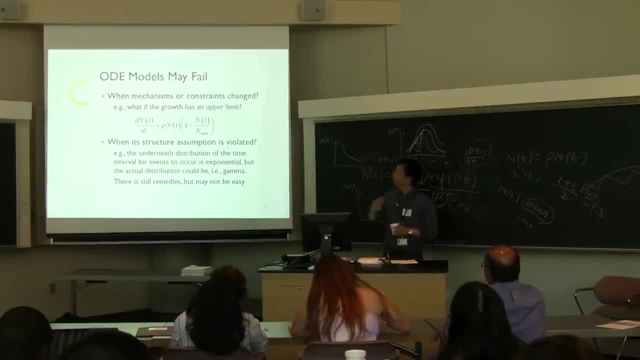 is that ODE model structure is subject to change. OK If in your experiments or problem. OK, you need to consider constraints or whatever. OK, if my time window is very short. what I care about is a very short time window, I'm OK. 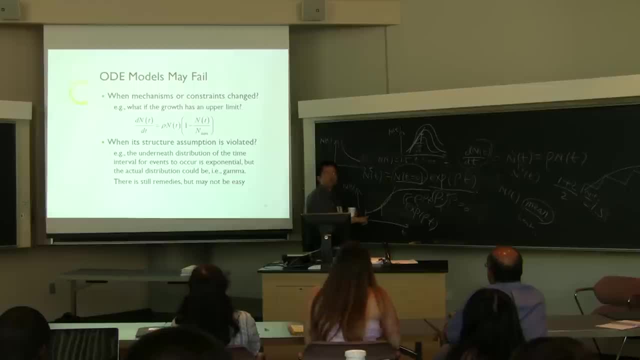 I can use that. I can use the exponential growth model because I know that saturation will never occur. OK, I can actually use the exponential. But once I know that in my experiments I will get saturation, then I have to take this into consideration. 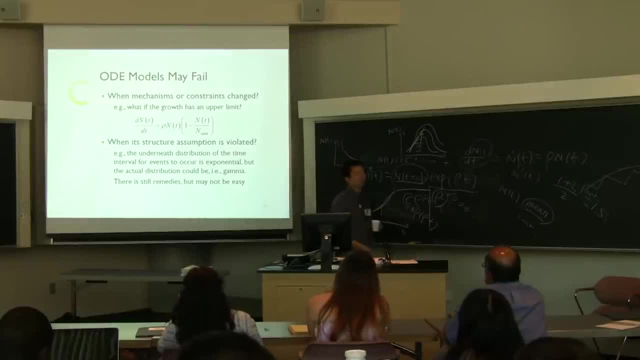 So that's how the ODE model does. OK, How they can. this is the way this model actually consider the saturation, by introducing one additional term here. So from here you can tell: actually, if N becomes N max- that's the max number you can get- the ratio becomes 1.. 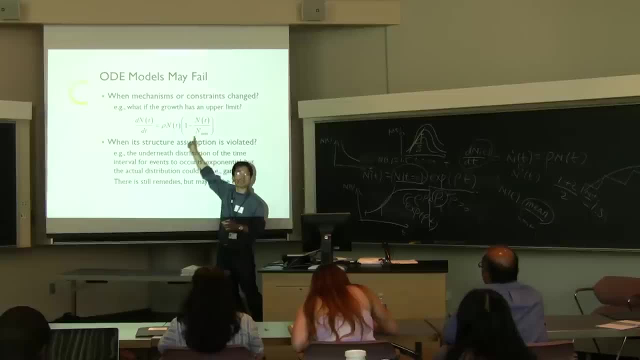 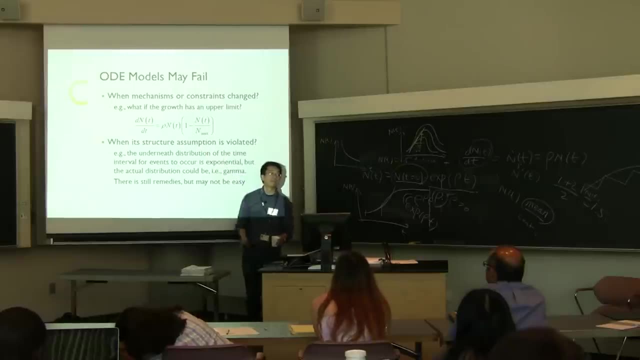 1 minus 1 becomes 0.. So right-hand side becomes 0,, which means the cell will stop growing. OK, That is the saturation right. So the rate becomes 0, means cells stop growing and you will expect to see a flat line, right. 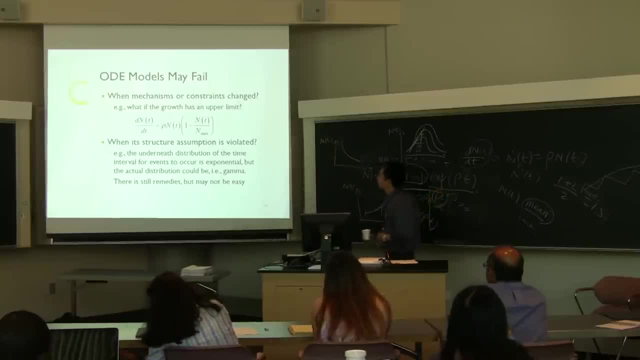 So the second one actually is the total number. a little bit tricky, OK. So once you use the ODE model, actually you also made another assumption, not an assumption in your experiments or data or whatever. Actually that's an assumption in mathematics, OK, 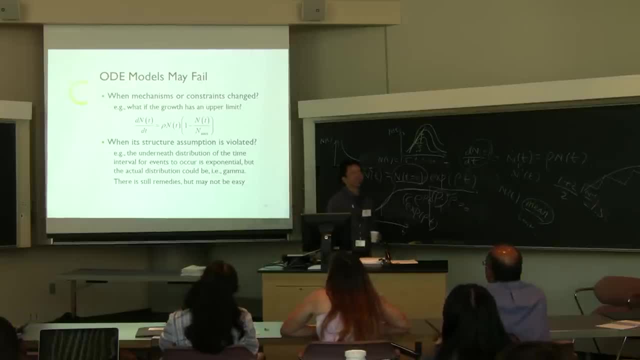 And it's actually easy to tell this implicit assumption. So the underneath distribution of the time interval for events to occur actually is assumed to be exponential. in ODE models, like what we just talked about, It's assumed it's an exponential distribution for. 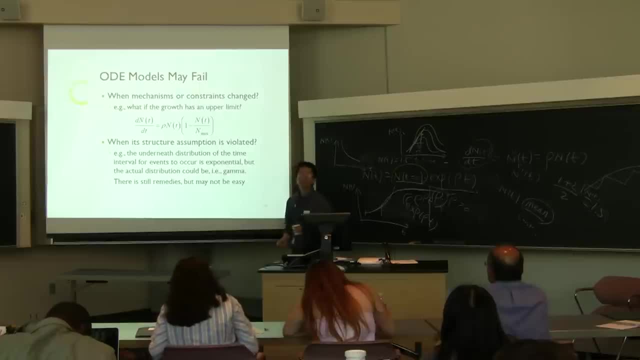 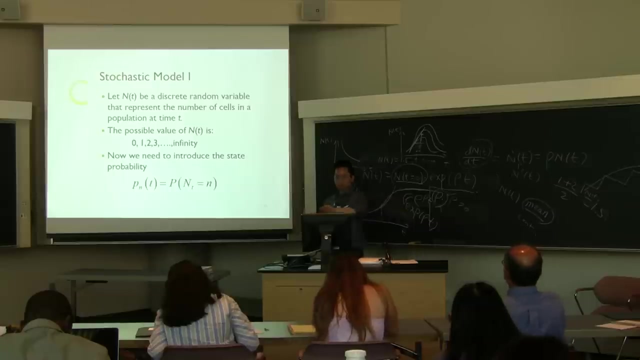 the time to event. However, once the time to event does not follow exponential distribution, you're getting. That's when the ODE model actually will fail. OK, I actually have an exam tomorrow to talk about this. Finally, I think I'm over time. 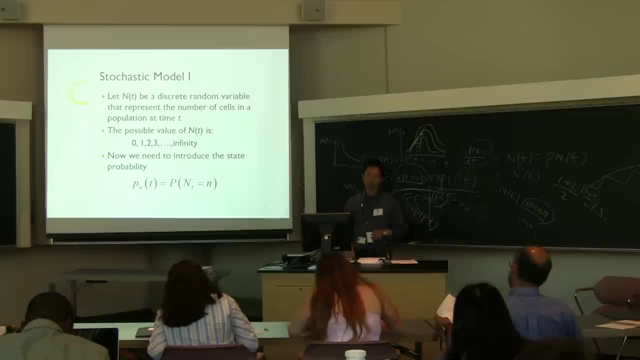 So, finally, let's just spend one minute to go through the stochastic model, because that's really not my focus. OK, because tomorrow we're going to spend a whole day to talk about ODE. OK, And Catherine will be the one who cares about the. 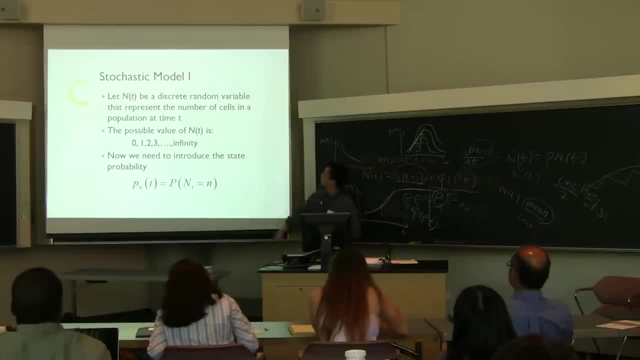 stochastics. OK, But the basic idea is that now, if I use the stochastic model, like I just mentioned before, I can actually directly model the number of cells. which means now I will model the integer. OK, I will get an integer for the number of cells. 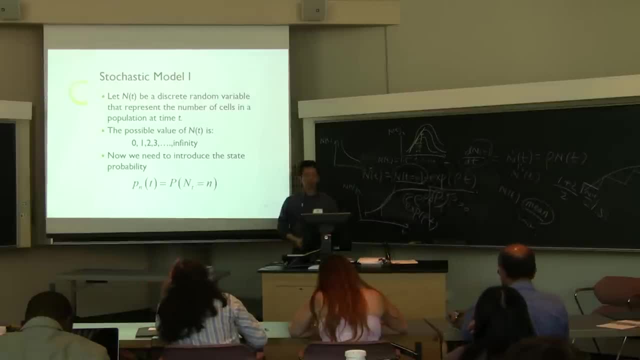 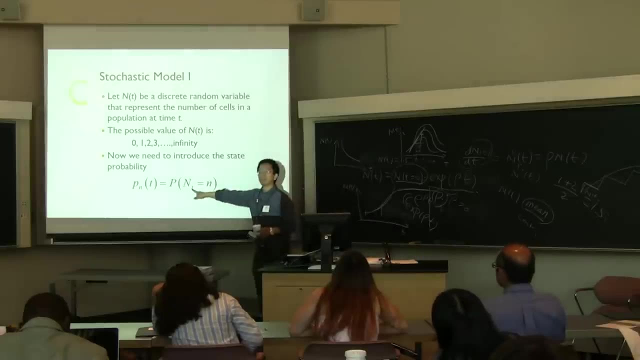 And basically the duration of the. this kind of model is based on the probability. OK, So, for example, at time t, what's the probability that the number of population is 1, is 2, is 3, is 4?? 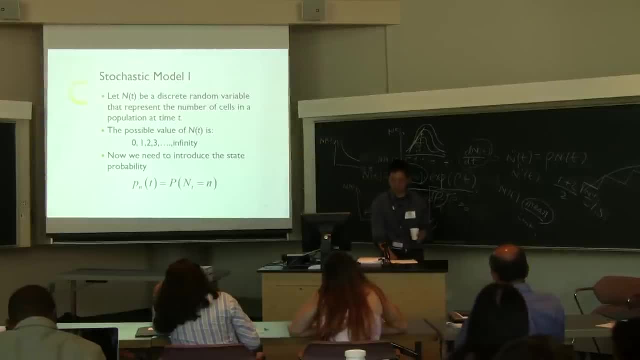 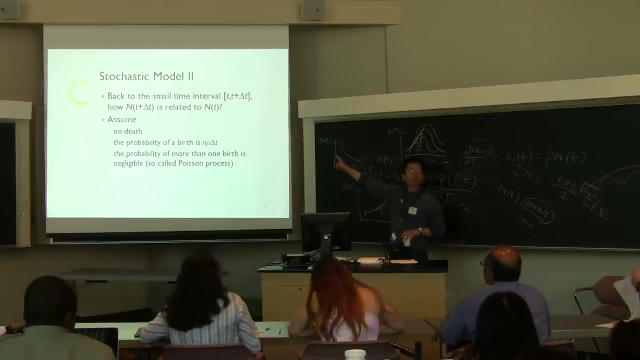 So once you have this probability, then you actually specify the whole population or whole model. So again, if you're interested, you can take some time to read the slides- and the basic idea is the same: that we actually look at the changes in the cell number during a small time. 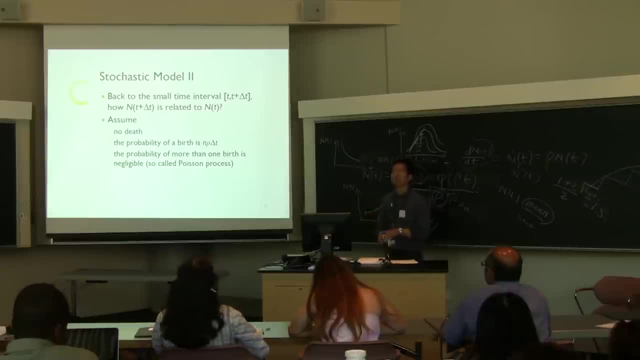 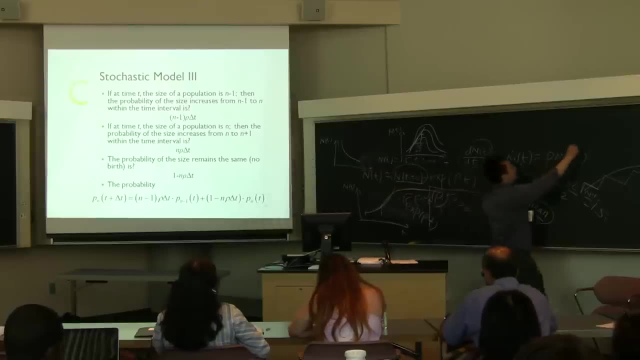 interval At time t- OK, We still start from there. OK, But how we deal with it actually is a little bit different. For example, if I have n cells at time t, OK, I can actually have only one duration. 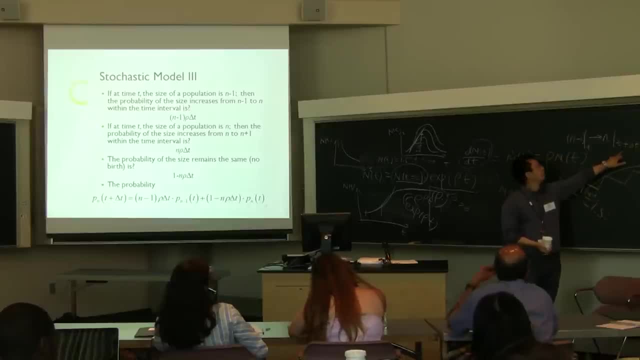 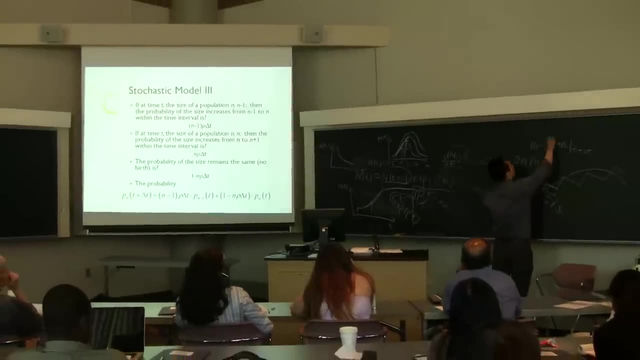 So if I have n number of cells, If I have n number of cells at time t plus 30, I can start from n minus 1 cells at time t, right, And then if I have n 1 cells, then I start from here and get. 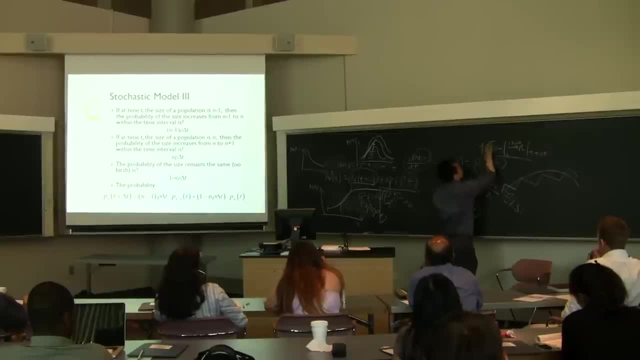 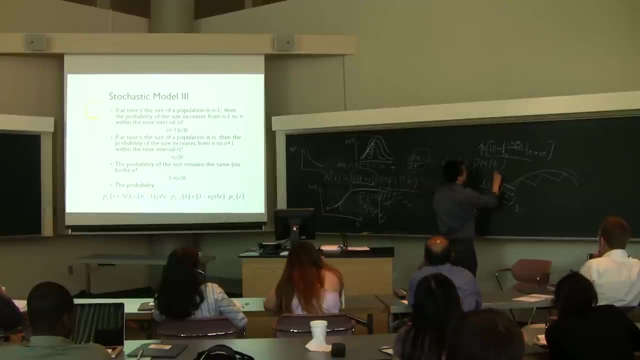 here. So then we calculate what's the probability of this event. Same thing If I already have. sorry it's sort of messy, but can you read: If it's already n cells at time, t, then after a time interval. 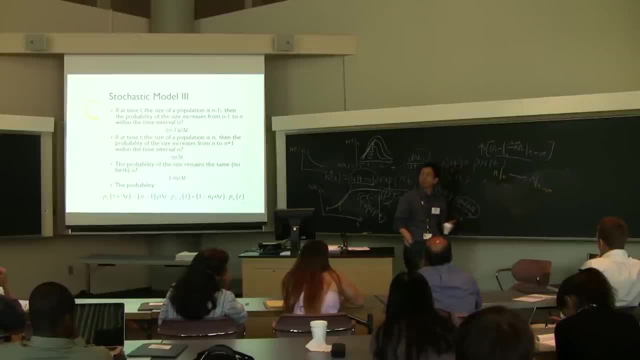 the cell number can remain the same. OK, So I also calculate this kind of probability. OK, So what's the probability that the cell number remains the same? So after I calculate the possible probability and then I can form this, OK, 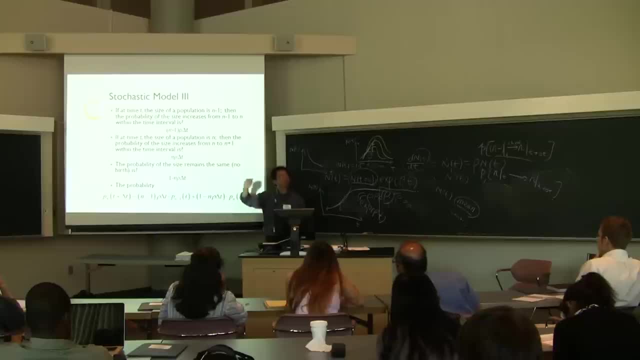 OK, I can form this kind of sort of equation. OK, So I calculate different ways to get this same number And then I add the probability together and then you get the total probability. That's all. So that's actually the idea behind. 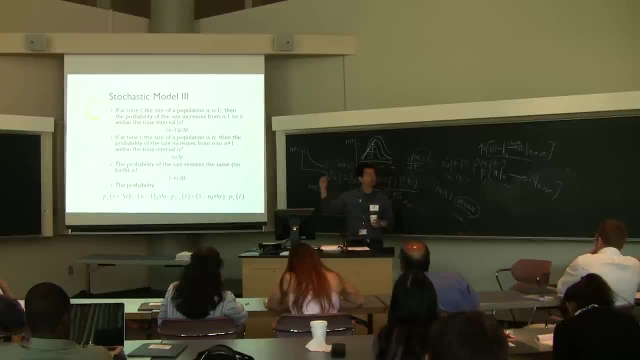 Although mathematically it's a little bit more tricky, OK, But the idea actually is simple, OK. So I think I'm going to stop here and see you in the software room.